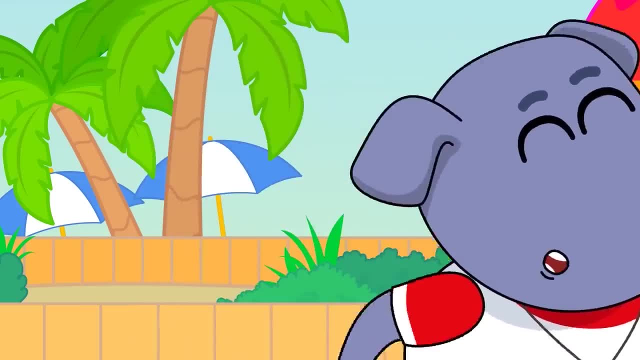 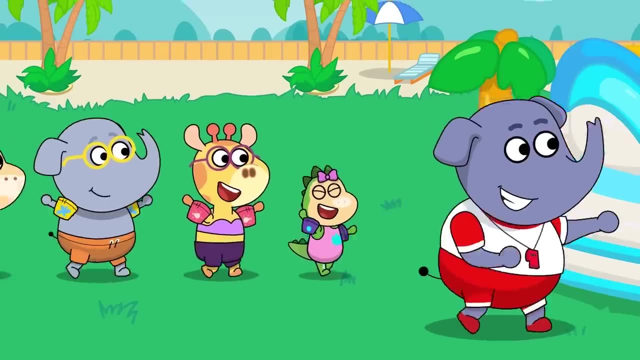 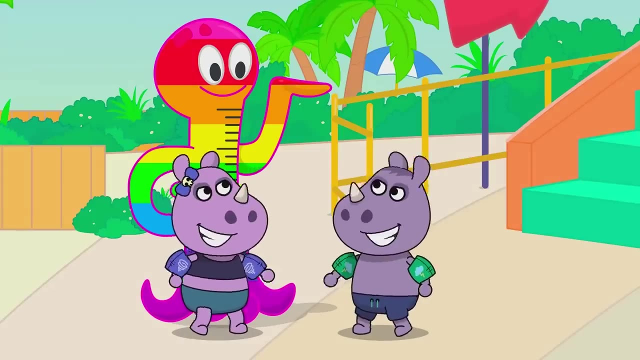 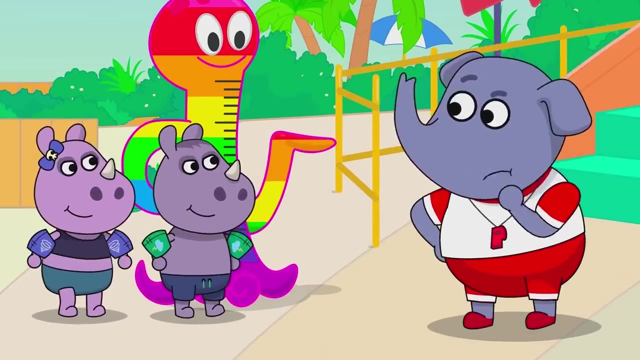 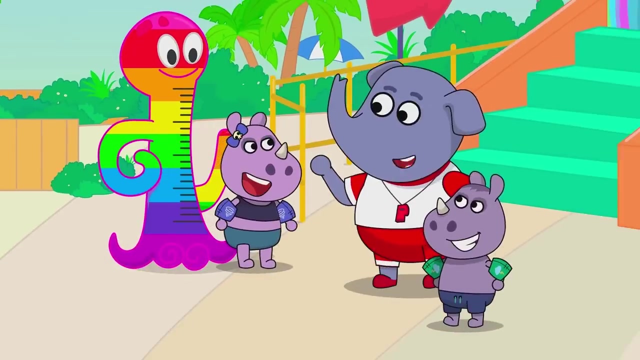 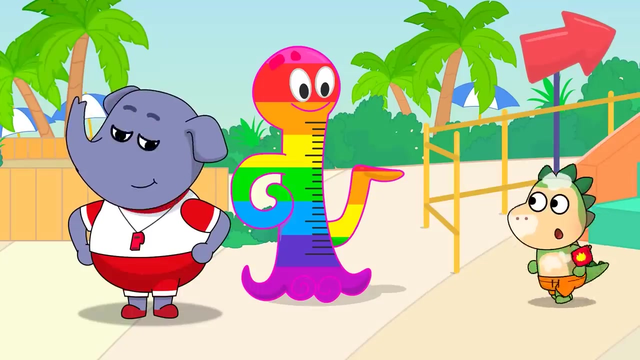 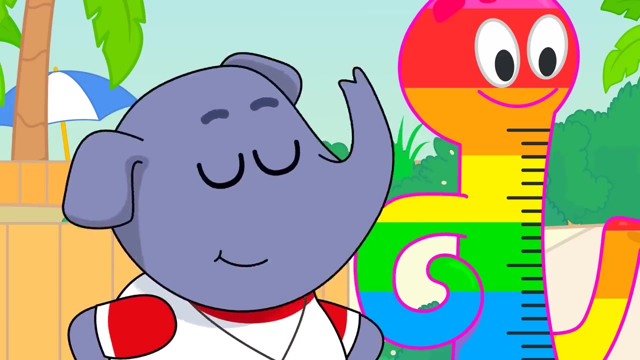 Oh no, Don't worry, kids, You can take the smaller slide. Yay, Wait a second, Let's see if you're tall enough. All right, Go on. Yeah, No way. Hmm. Hmm, Seems okay, Go on. 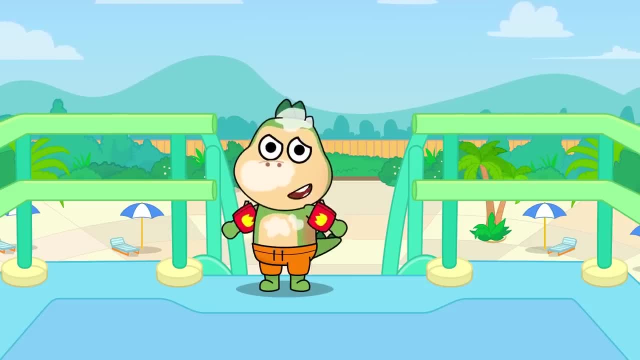 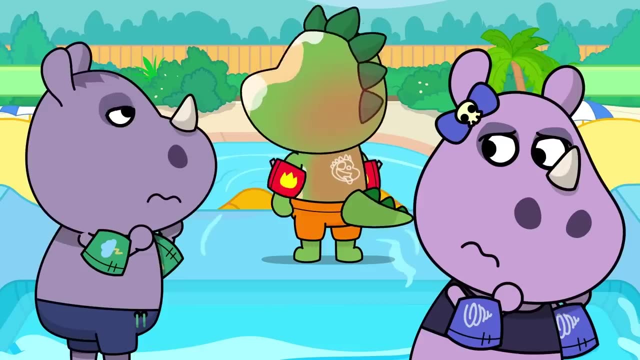 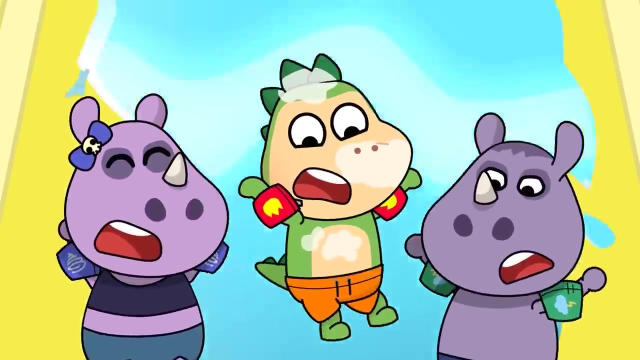 What are you doing here? What are you doing here? It's too high. Oh, Oh, Oh, Oh, Ugh Whoa, The teabag is fried. Whoa énd, Whoaénd, Whoaénd. 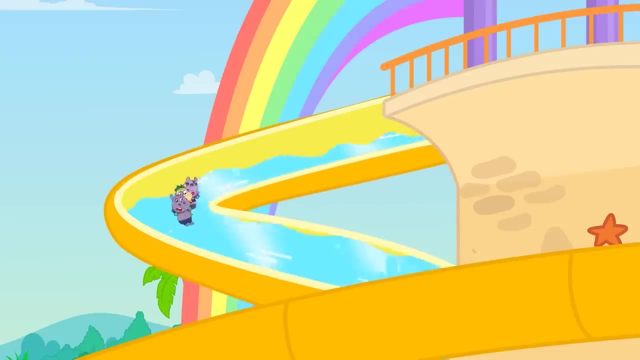 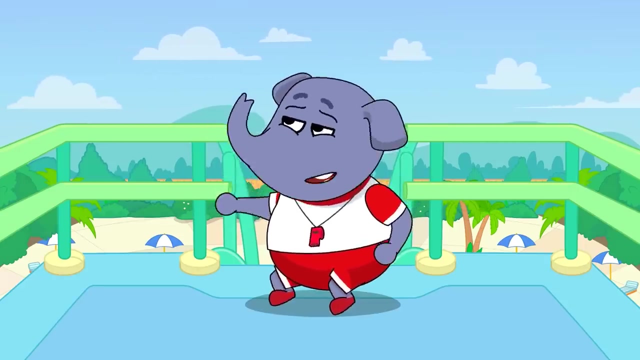 Whoaénd, Whoaénd, Whoaénd. Oh, I'm so cold. Whoaánd, Whoaénd, Really cold. WhoaND, WhoaN, Wow, WhoaND, WhoaND. 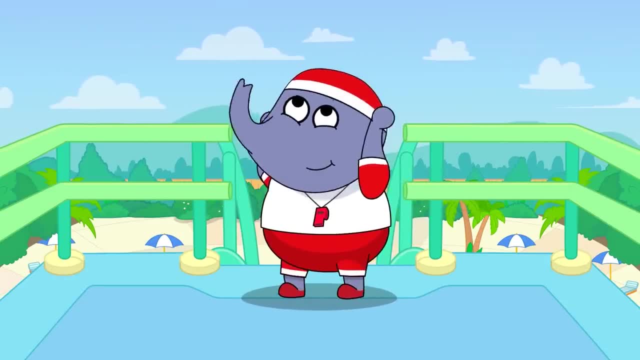 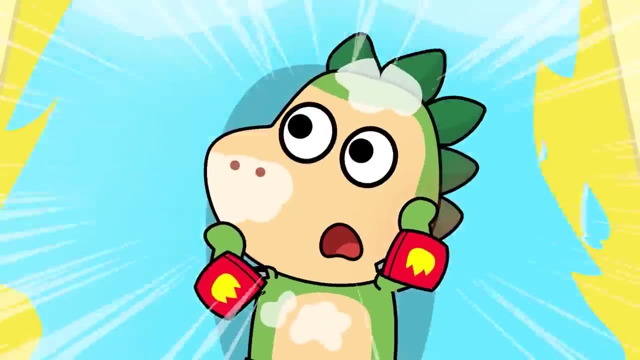 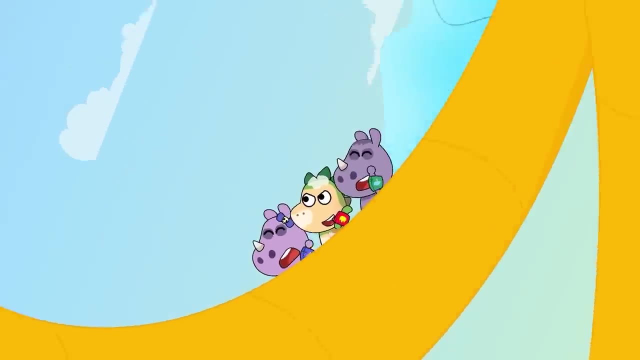 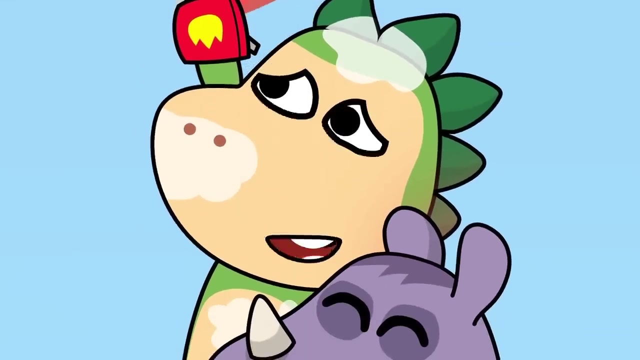 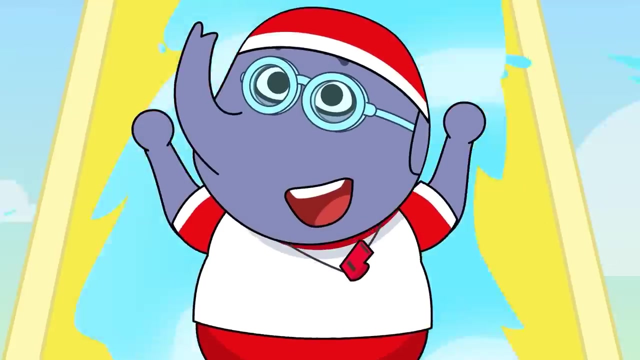 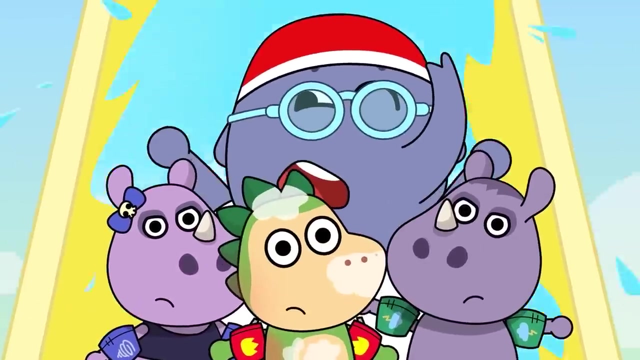 Oh boy, What's that? It's a공, It's a. Oh, it's hot. What Tide. I have an idea Now what I don't know. Get ready kids. Yay, Welcome back. That was dangerous. How did that happen? 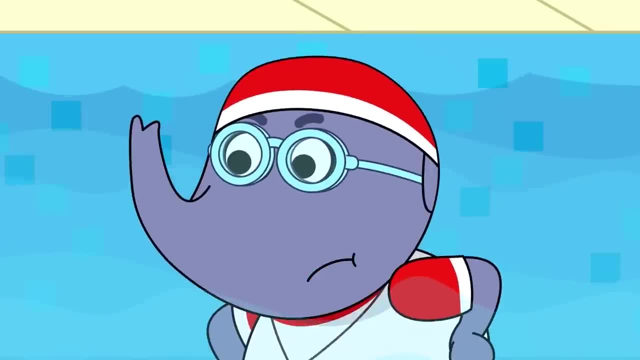 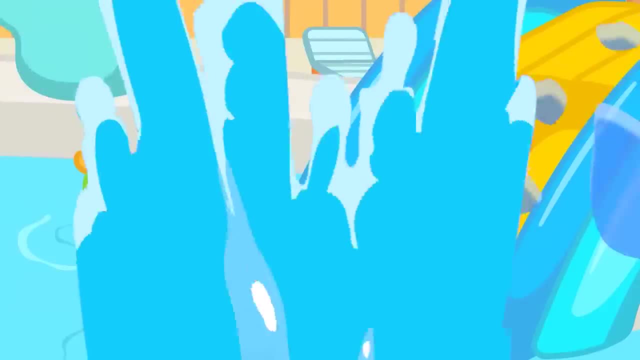 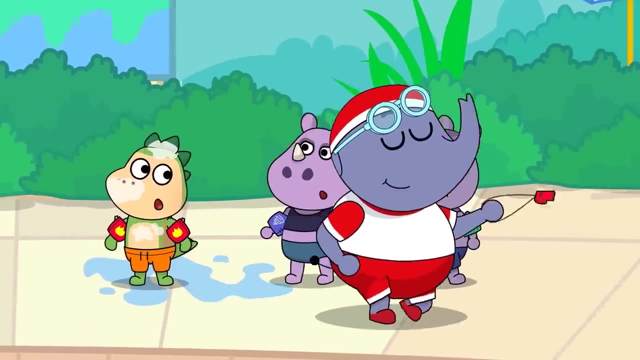 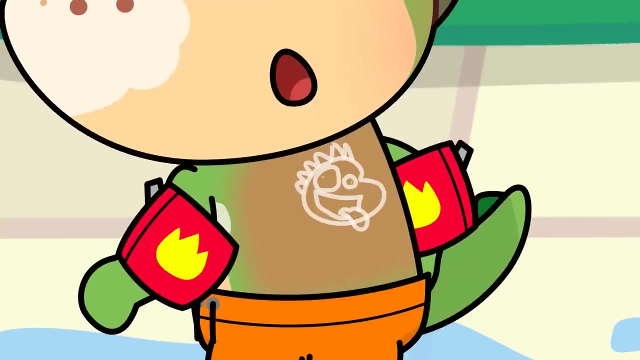 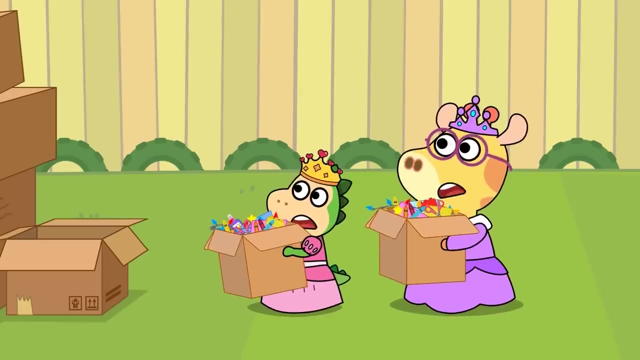 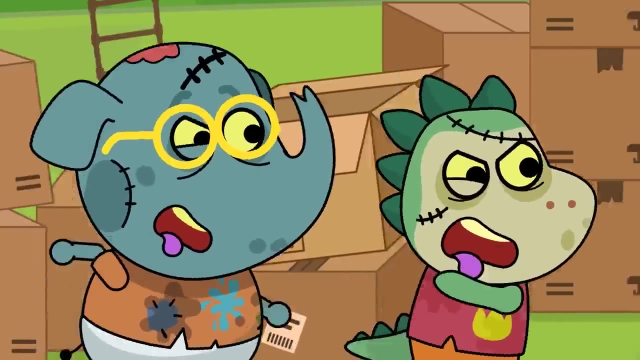 We changed the height of the slide. measure You what? Aha, It's time to learn more about safety. Hey, No splashing, Remember kids. Safety first Sparkle. Those boxes are blocking our way. I'll protect them. 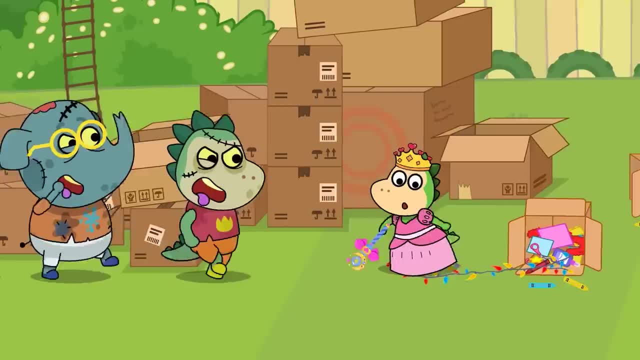 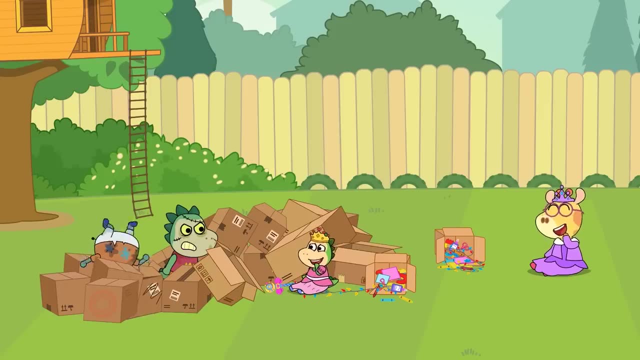 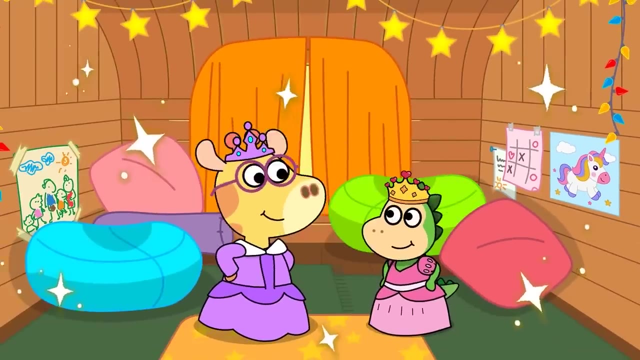 Box on me back. Oh no, Sparkle, We're trapped here. We're trapped. Oh, We seem hungry, Let's get lunch. How are we going to get down? We're trapped up here. Look, No way You think you can trap us with no lunch. 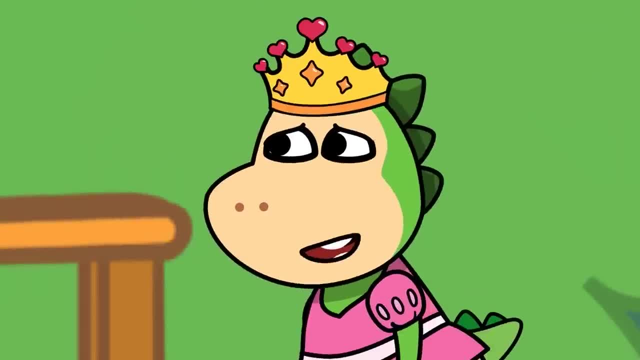 This is it What, Sparkle? You don't know the way, Come here with those treats, What You think? you can trap us with no lunch. This is it. Why are we trapped here, Sparkle? We're trapped. 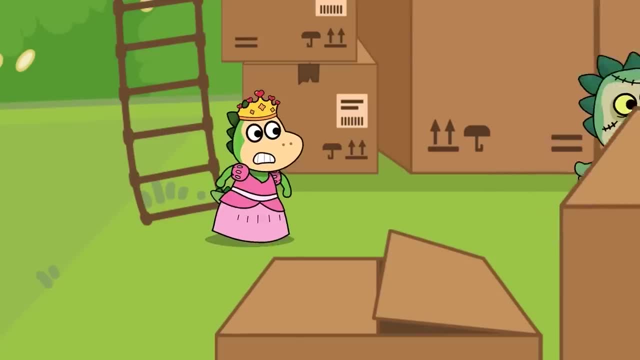 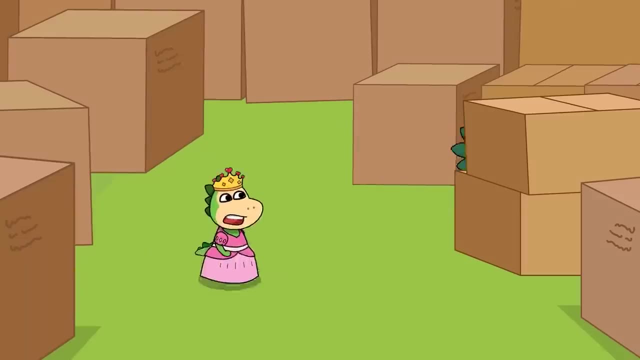 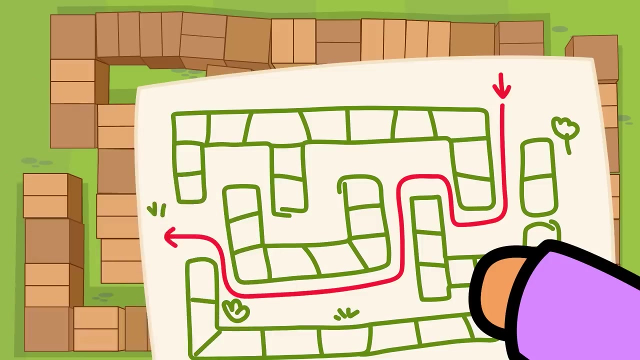 Look, Look, We're trapped. What, What Sparkle, What? Why are we trapped here? What? Ha, ha, ha, Ha, ha ha. Oh, Huh, Wow, Huh. Hmm, Okay, I think I almost got it. 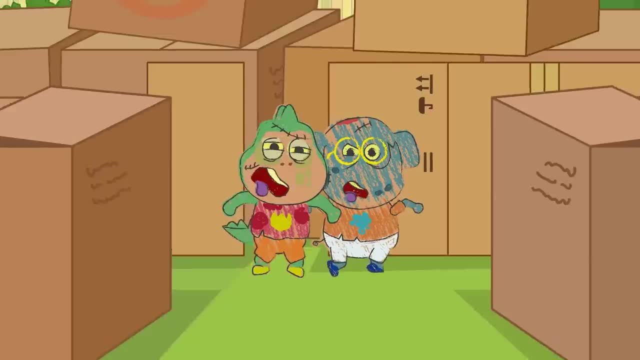 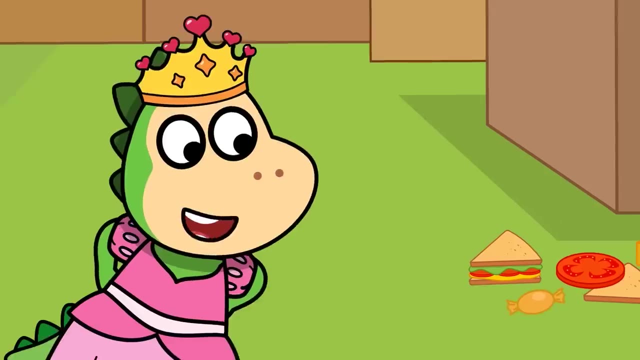 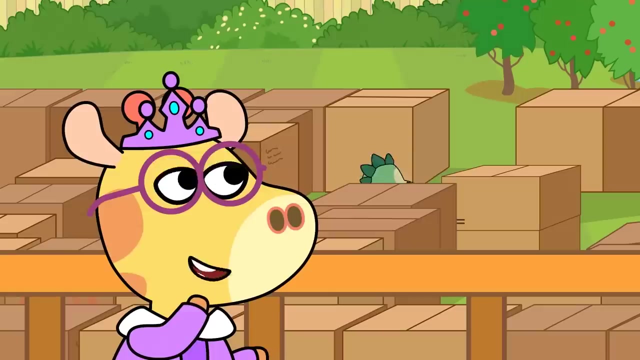 Spike Models. Where are you? Aha, There you are. What? That doesn't look like Spike at all. Huh, Okay, now I got you. He, he, he, You're mine now. Spike just got out. Hee, hee, hee, hee, hee. 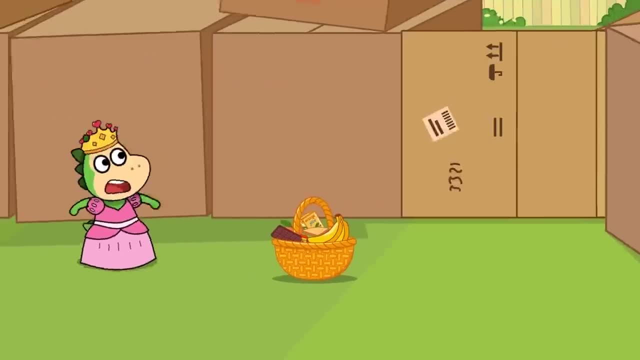 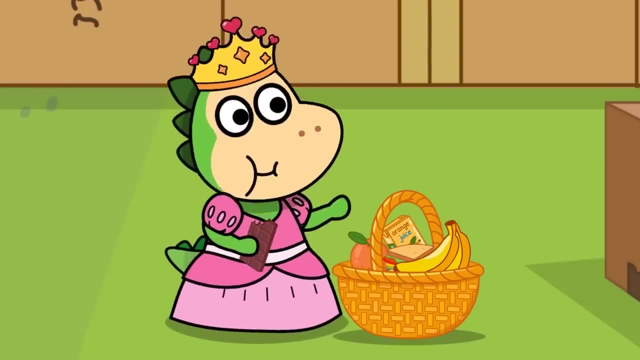 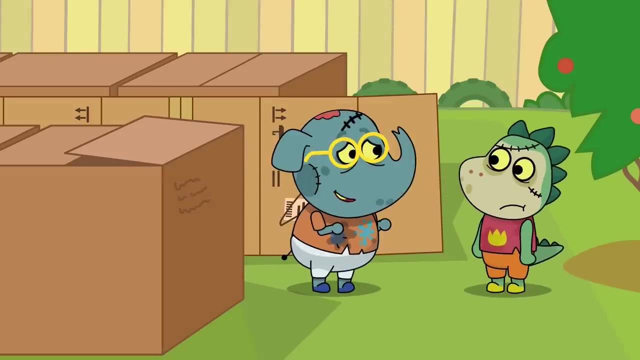 Ah, I've lost him, Huh Hooray. Oh no, I think I've lost. Why did you leave the fort? Hee, hee, hee. I was looking for you. I won The fort. mystery is solved. 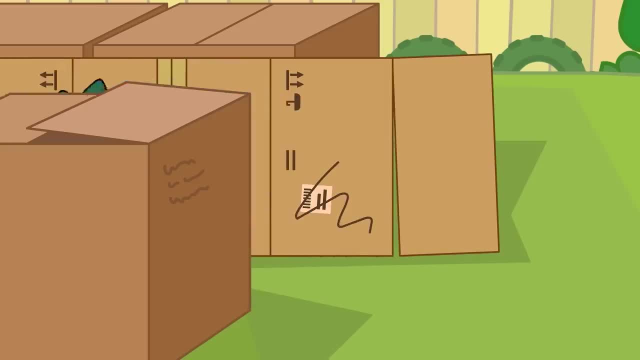 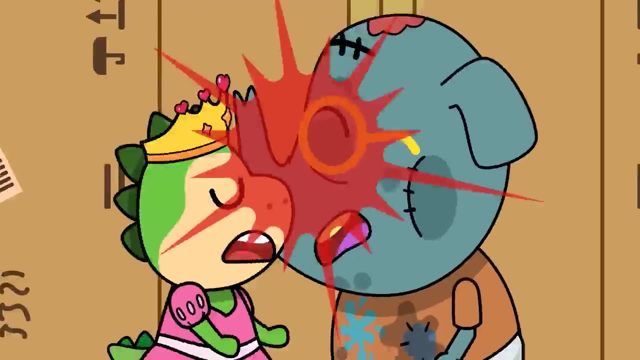 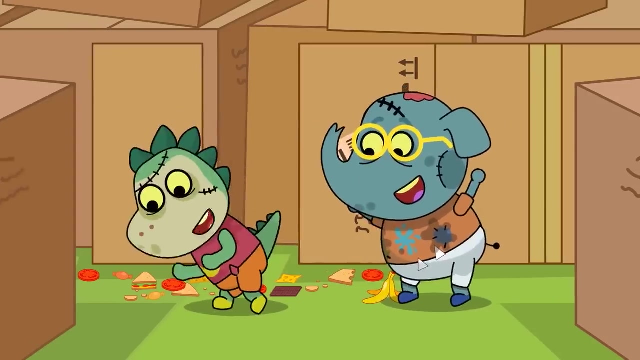 Oh no, We have to get to the lunch tree. Where did you leave the lunch tree? I don't remember. Huh, Ah, A zombie, A princess. Follow the tree Quick, Hmm, Delicious, But don't eat them all. 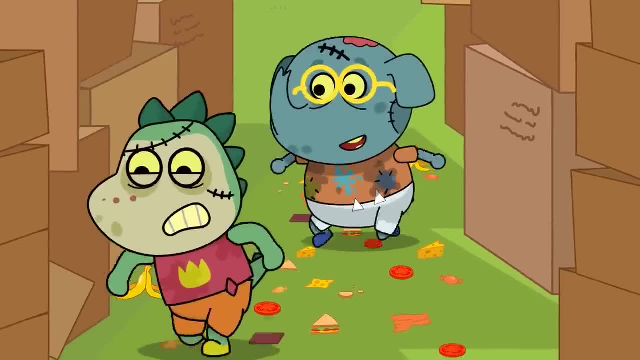 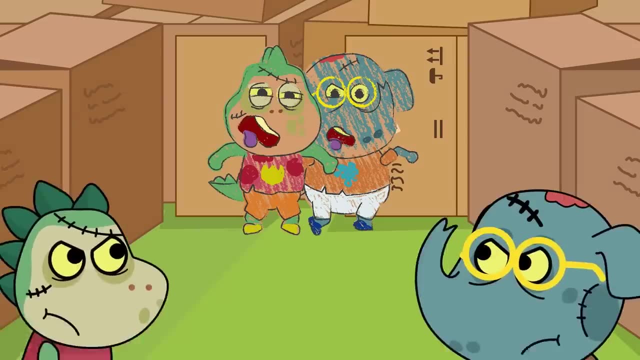 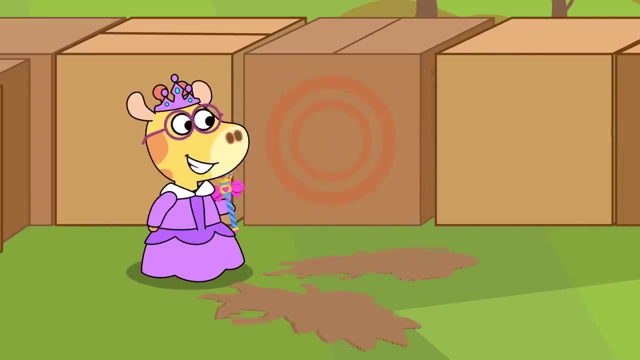 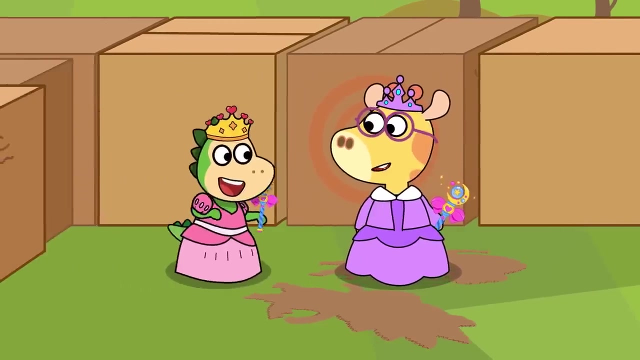 Ah, Pom's going for the trees. Oh no, They're just behind me. Hmm, Where did she go? Whoa, Ah, Hee, hee, hee, hee, hee Sparkle. Hey, Let's go before the boys come back. 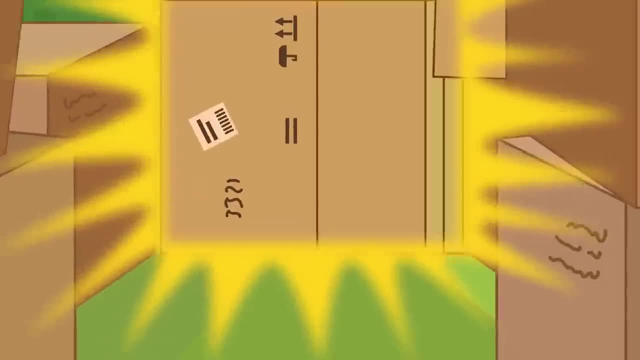 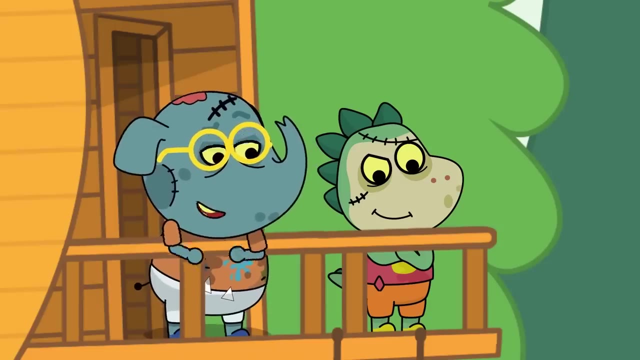 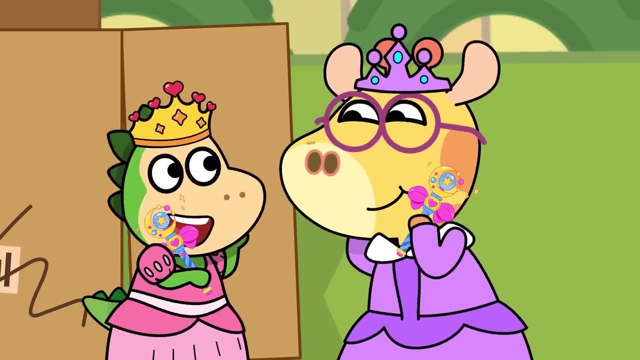 There's the exit. Yay, We did it. Oh yeah, Huh, Now we have the treehouse, But this palace needs two princesses. Ah, Ha, ha, ha, Hee, hee, hee, hee, Huh. 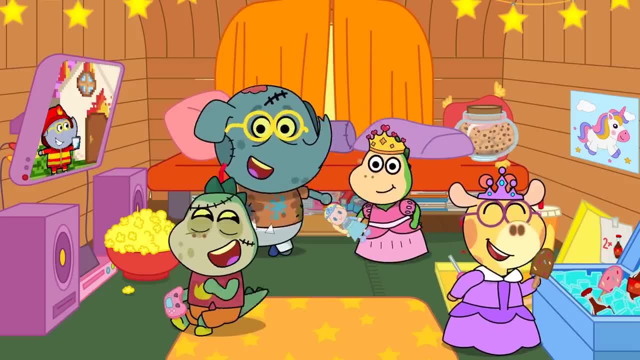 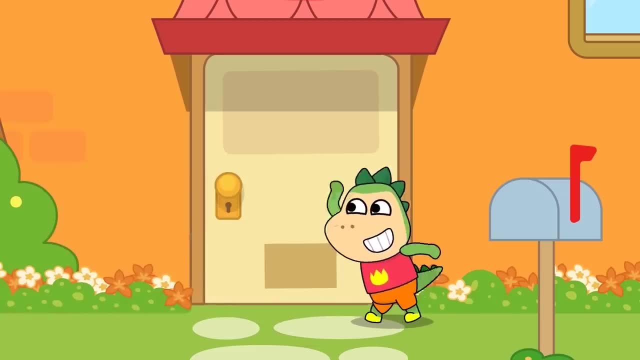 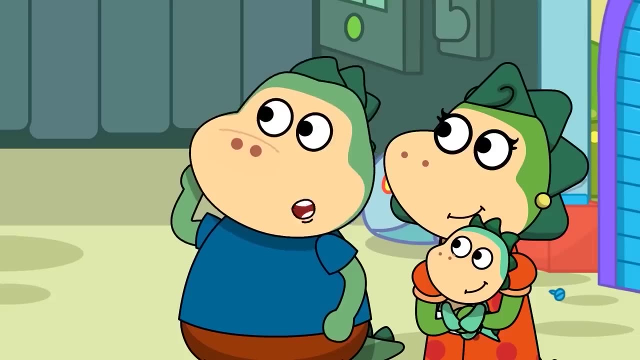 Hee, hee, hee, hee. What's all this mess? Ha ha ha ha. Mommy Daddy, What is it? Spike? Professor Roar is having a yard sale. Hello, Professor Roar, Is everything for sale? 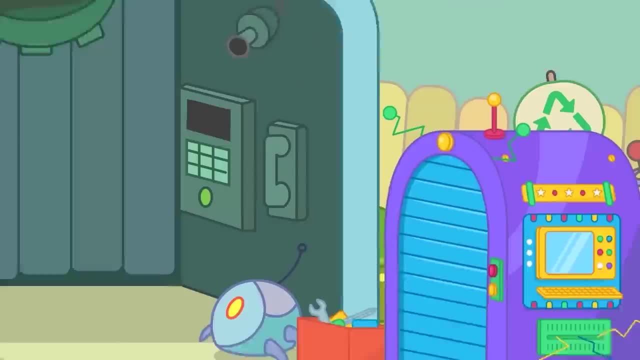 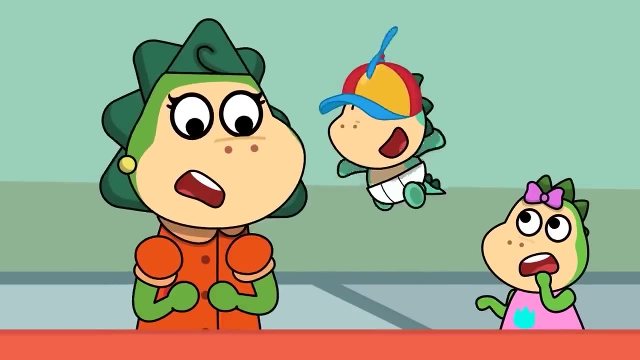 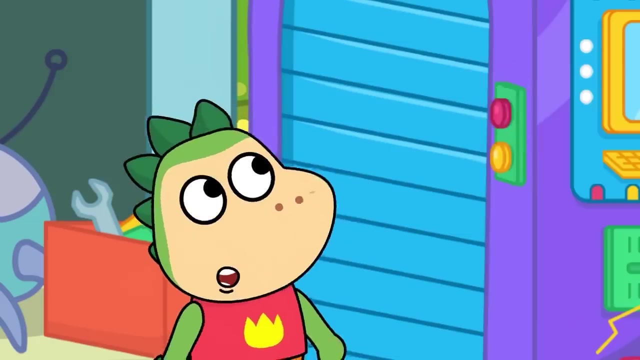 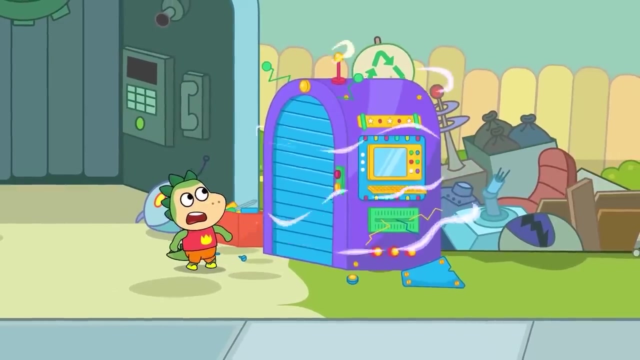 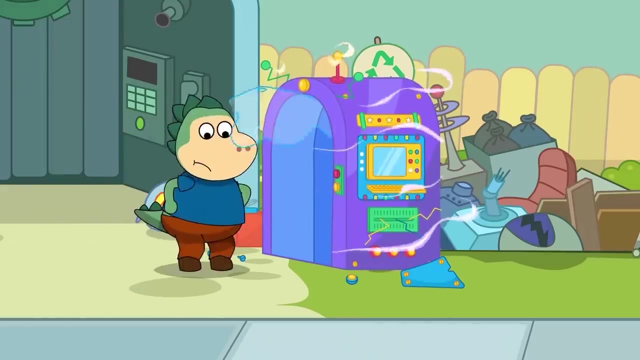 Oh, welcome, Yes, everything but the collar booth. Ooh, Ooh, Hmm, Huh, Wow, Wow, Wow, Hmm, Hmm, Huh, Spike, You heard, Professor Roar, That's not for sale, Ah. 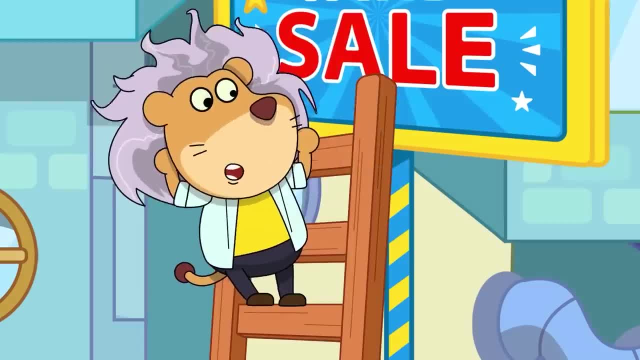 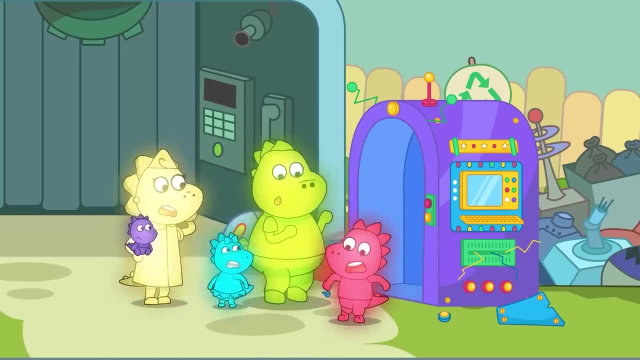 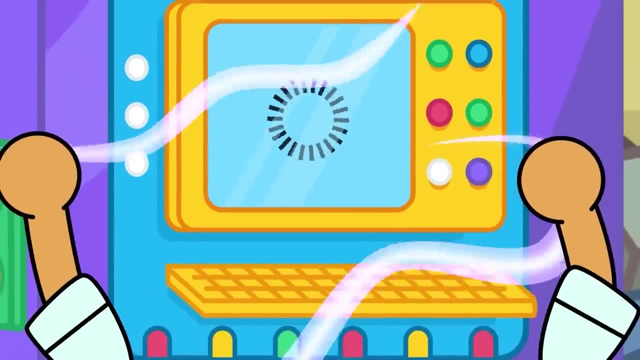 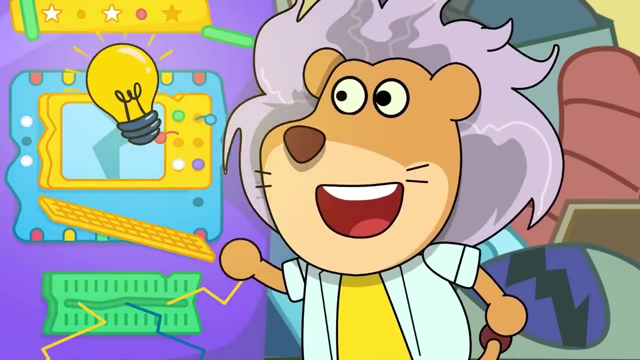 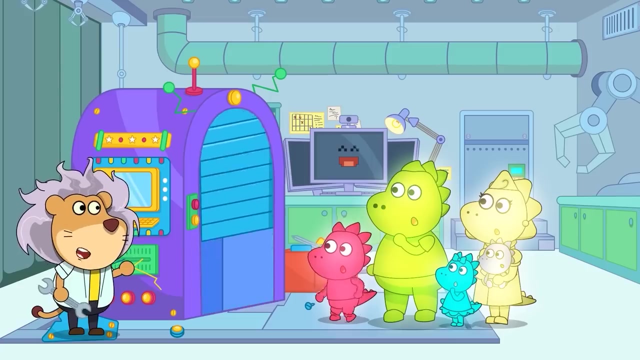 Hmm, Honey, No, Don't go in there. Ah, Ah, What happened? Let me fix it. Oh no, It's broken. What are we gonna do now? Aha, This should do it. Wow, This will change you back to normal. 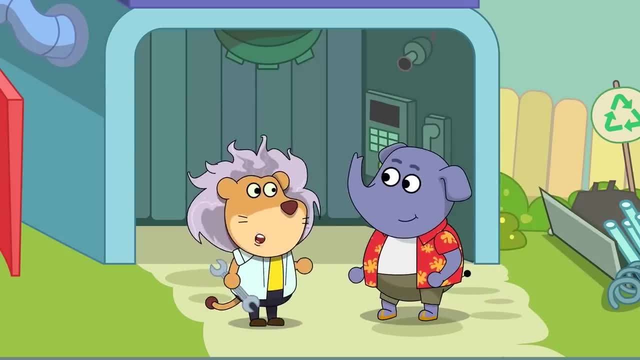 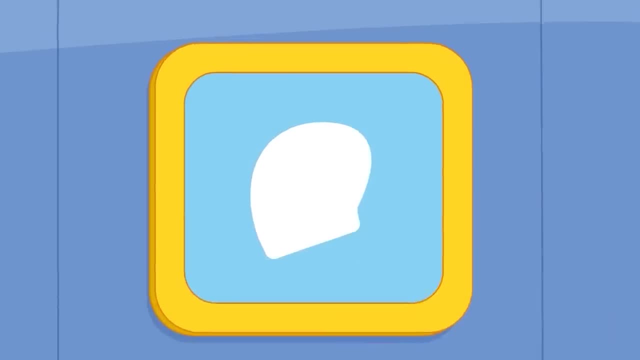 Are you here, Professor Roar? You won't believe what just happened. We just had a little fun. We just had a little fun. We just had a little fun. Have these squares by color to find the exit. Have these squares by color to find the exit. 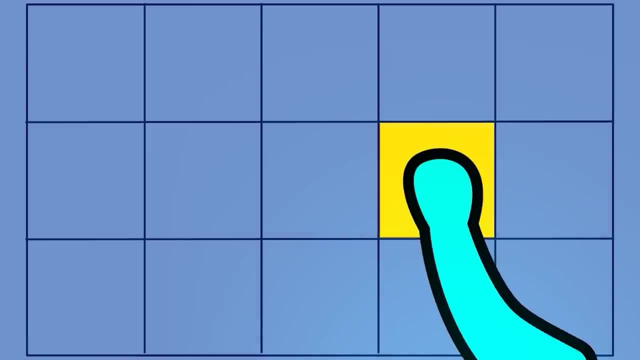 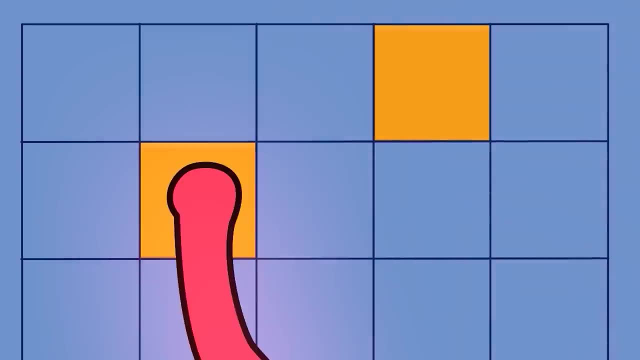 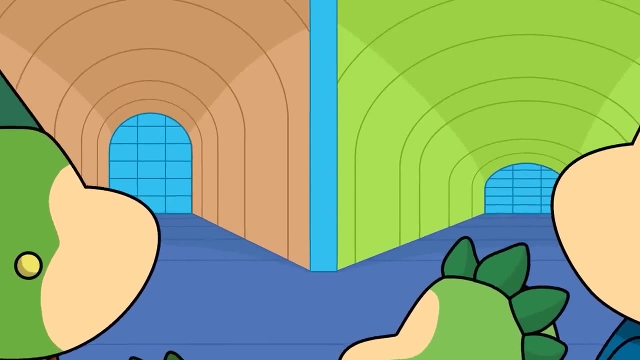 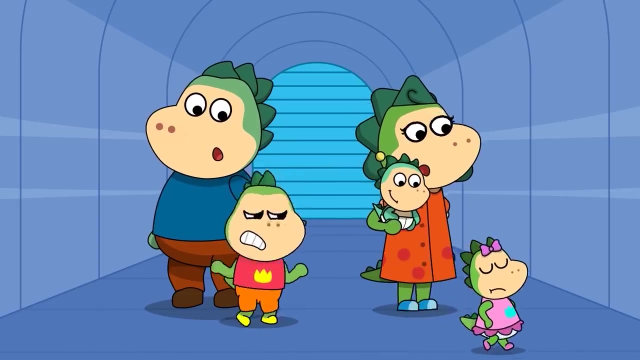 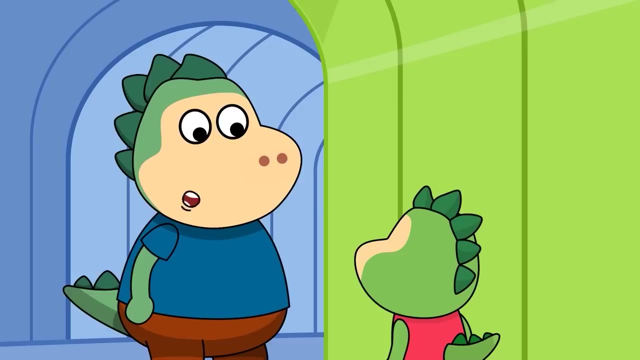 Hmm, I go first. Oh, Error, Error. One more chance. Hmm, Hmm, Hooray, Let's go right. No, let's go to the left. Huh, Look Daddy, What color should it be? 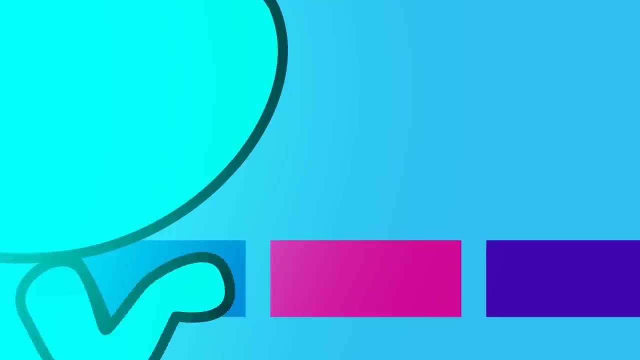 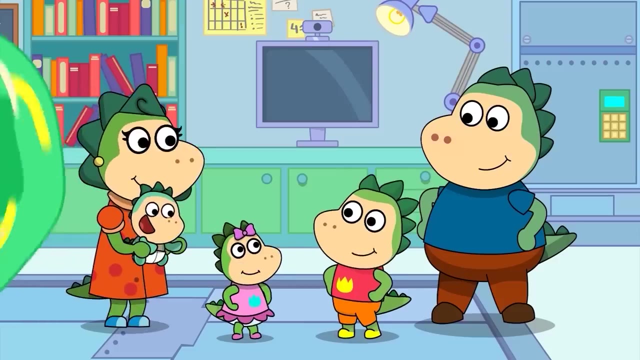 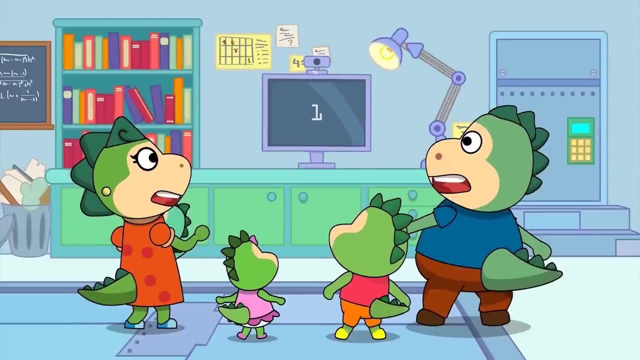 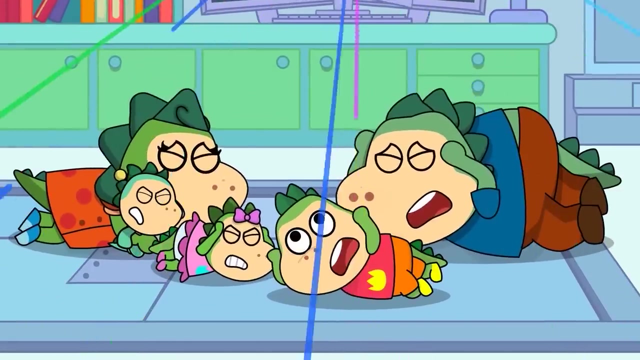 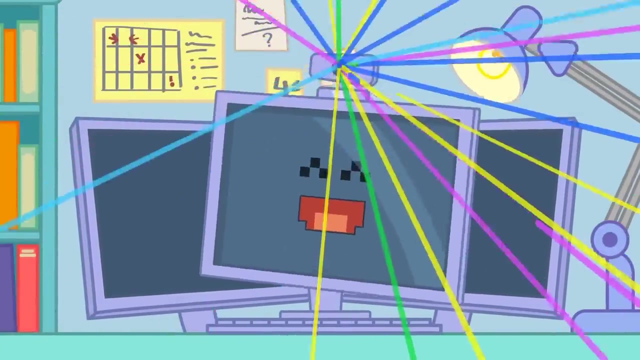 What color should that be? We are back to normal. Hooray Includes detected Three, two, one. It's so crazy. Get down What happened. It went crazy. It's out of control. Quick, help me find the right plug. 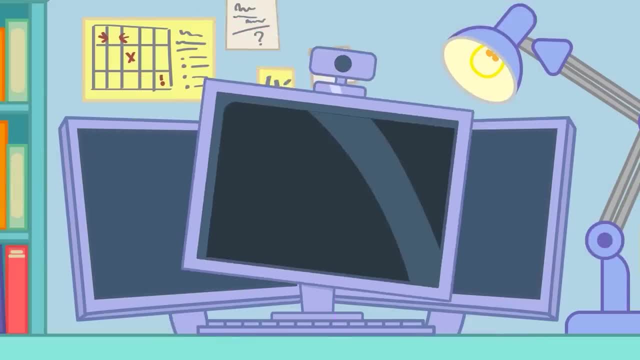 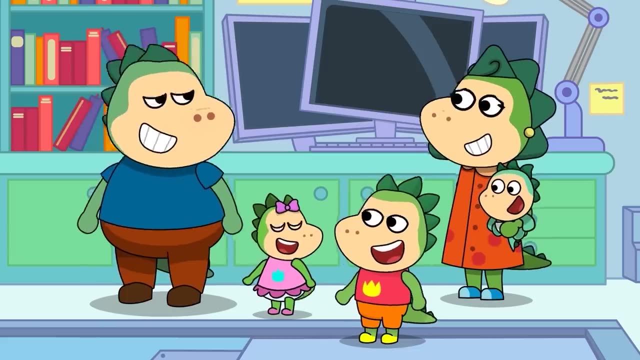 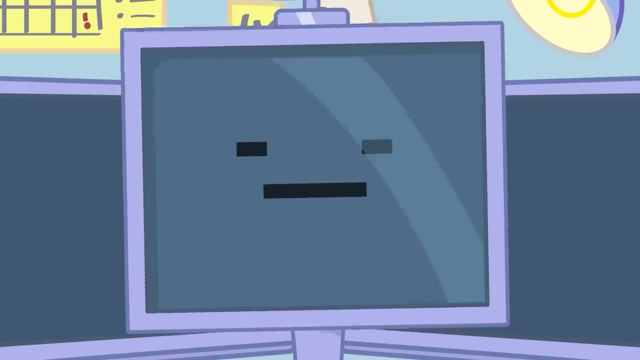 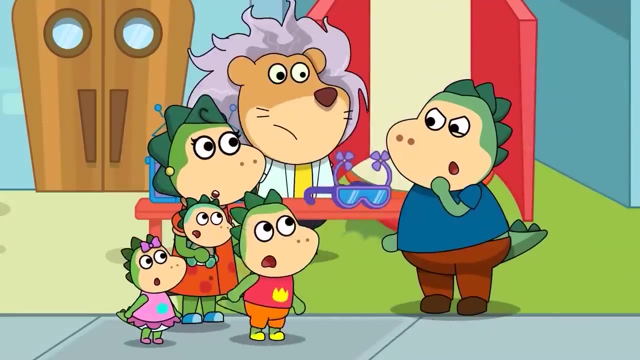 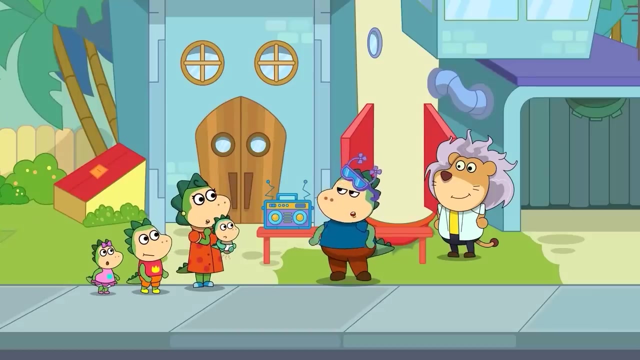 Well done, Spike. Now let's see if the computer works again. Let's hope for the best. Yes, it did. How can I help you today? Yes, I'll take this one. Are you sure? Sure What could happen. 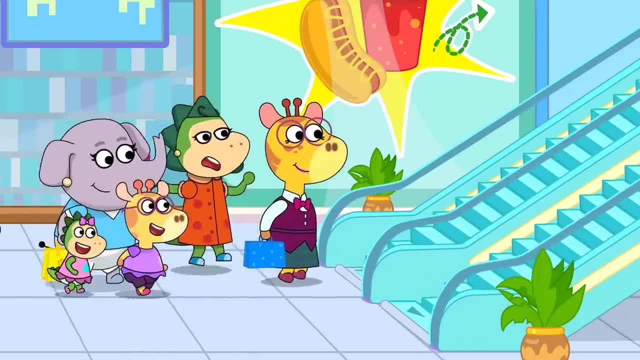 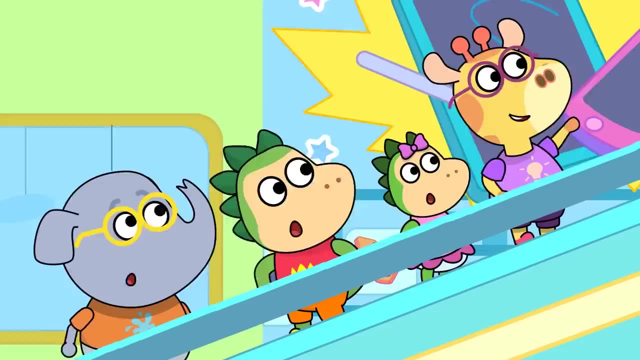 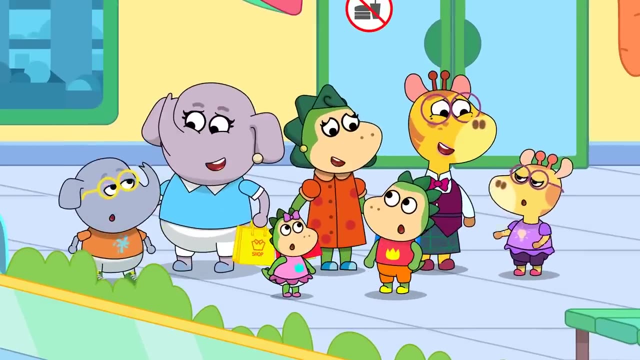 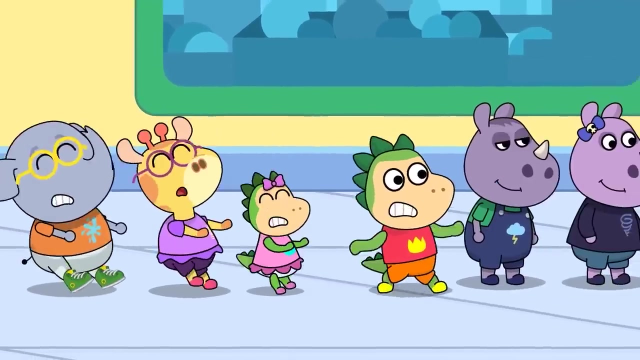 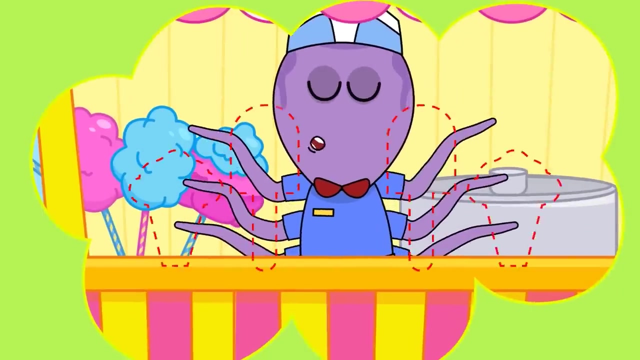 Kids, no running, Everyone Get your cotton candy Candy, Mommy, Mommy, Please, please, can we buy one? Alright, okay, But that's your candy for the day. Oh no, There are too many people. I'm sorry, kids, No more cotton candy, Don't worry, there's enough for everyone. 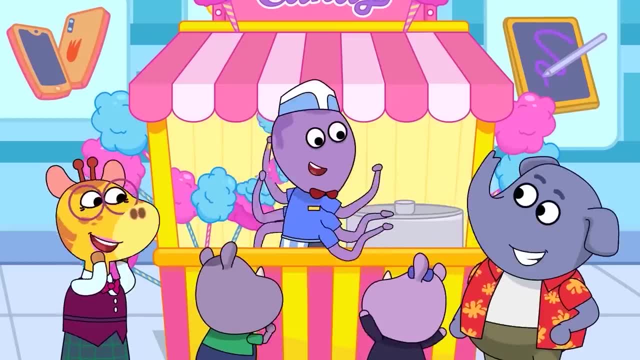 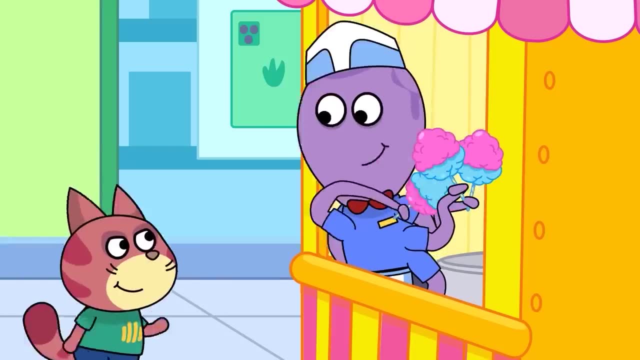 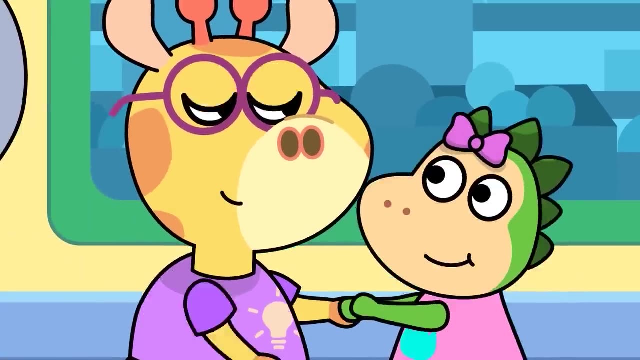 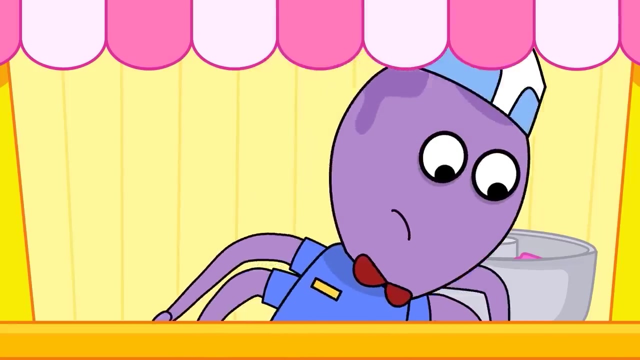 Come and get your cotton candy. Get them while they're hot. We're almost there. It looks like he's running out. Here you go. We're not going to make it. Yes, we will Enjoy. Four, please. You got it. Hmm, Are you all out? Here it is. 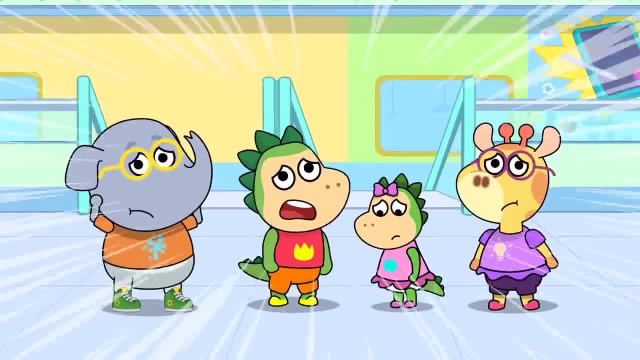 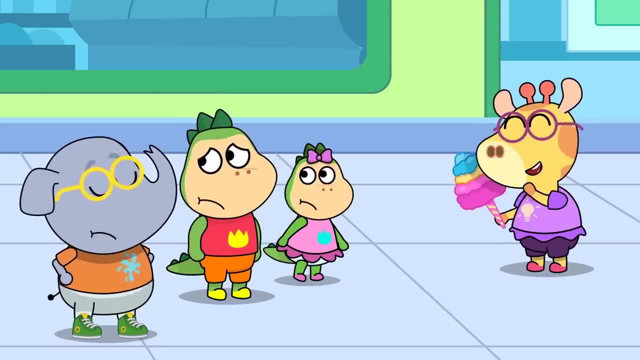 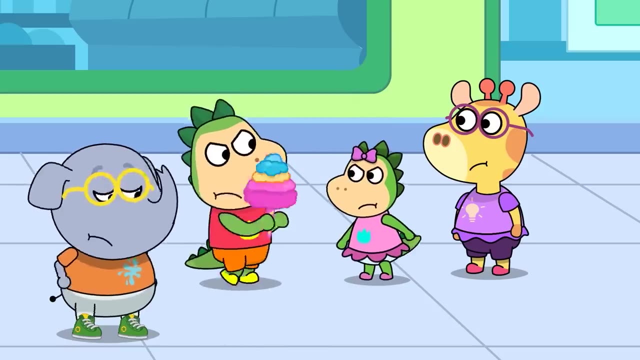 I have one left. Sorry, kids, I only have one left. We'll take the last one. What We want, some too. Poe, Here's an idea. Why don't we share it? I want the top. No, I want the top. They're going to drop it. 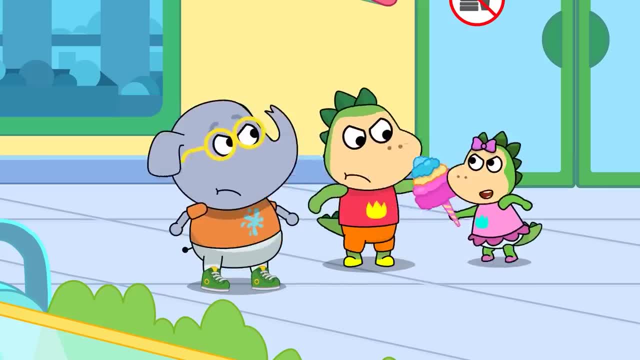 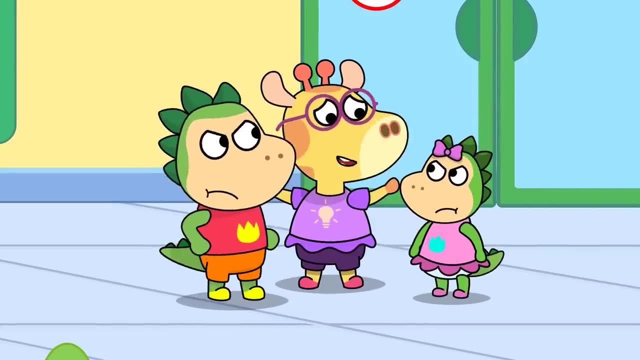 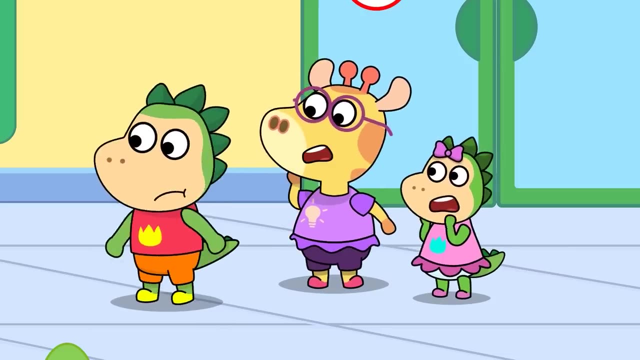 Please don't fight, We can figure this out. You take the bottom. No, you take the bottom. Let me hold it. No, Calm down, guys. We can split it evenly. Where did models go? And the cotton candy? Help me, Help Models, Come back. models. 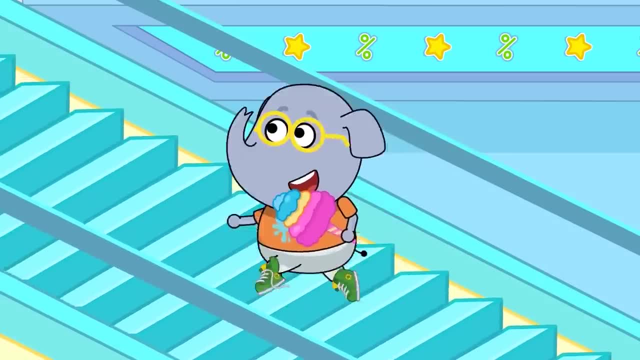 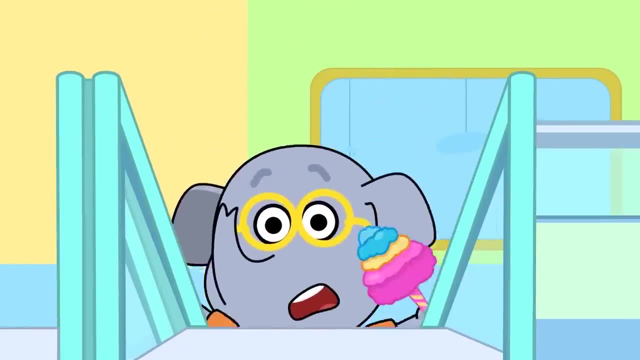 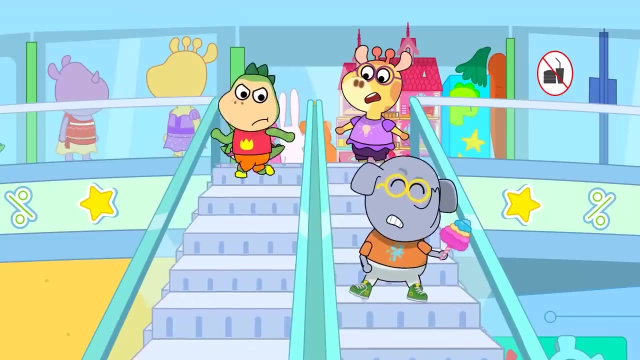 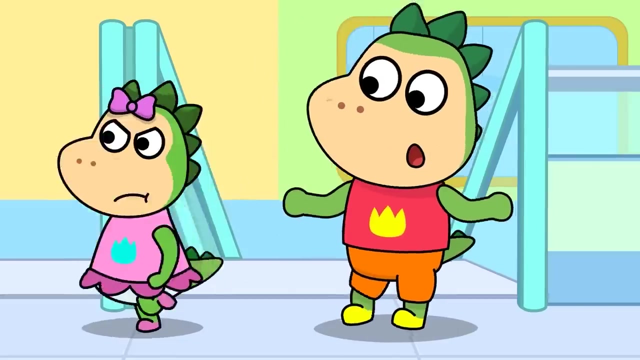 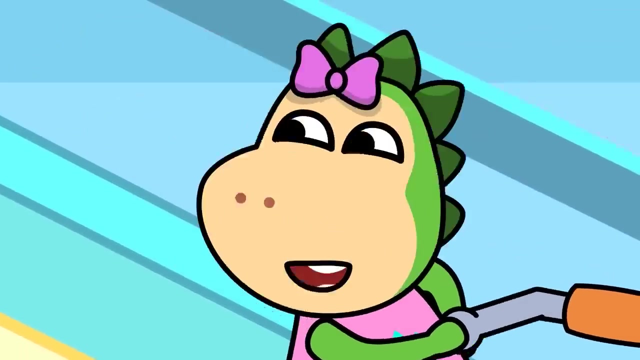 Hooray, Oh no, I'm stuck. Let's rescue that cotton candy. Huh Huh, Models, I'll help you. This is not working. That's going up. Come on, cotton candy Spike, help us. Okay, ready One, two, three. 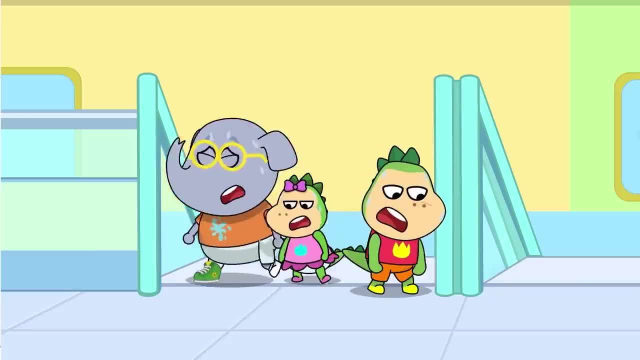 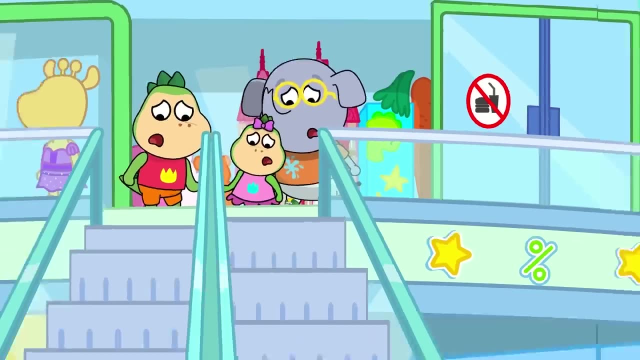 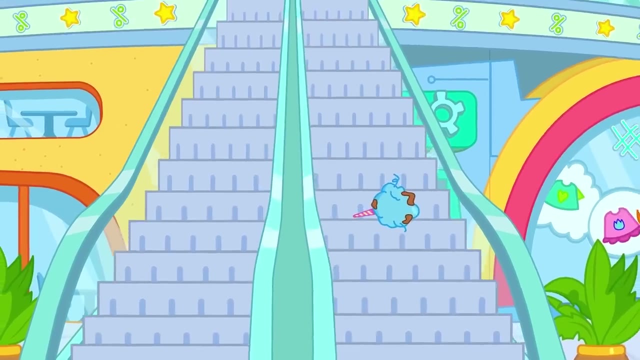 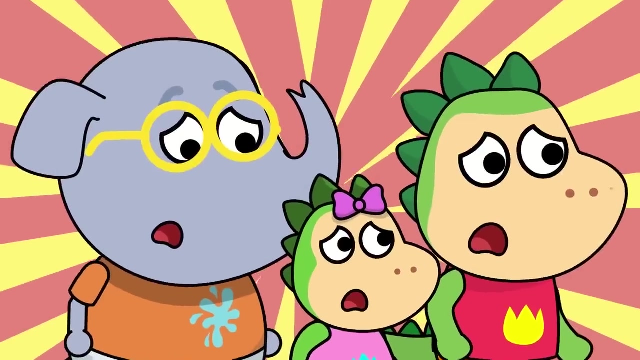 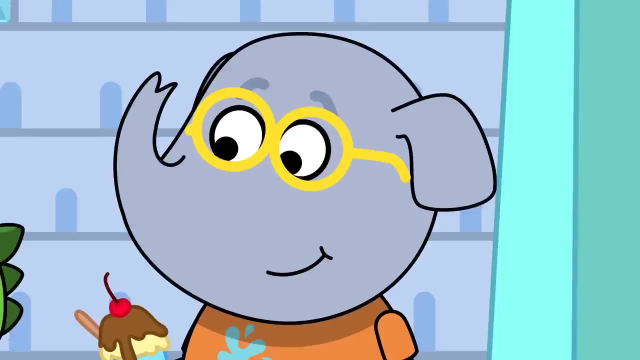 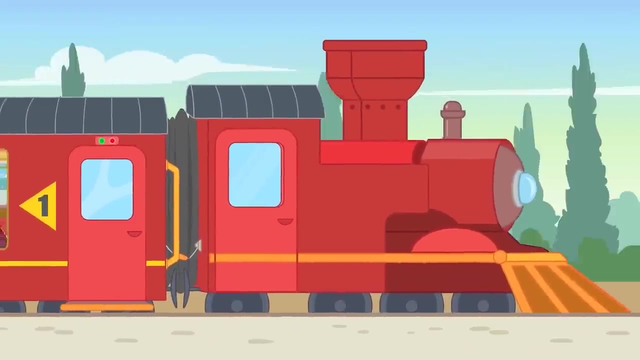 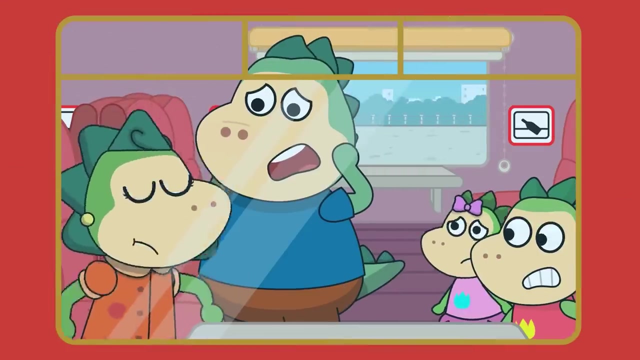 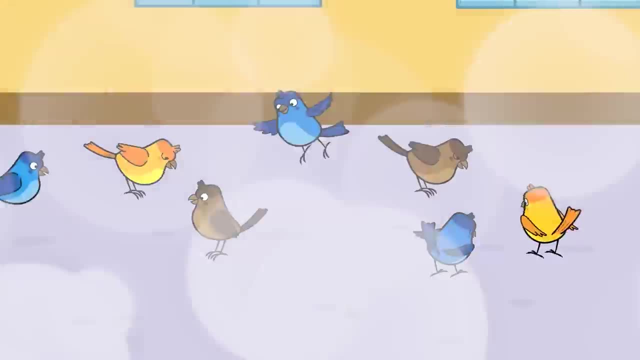 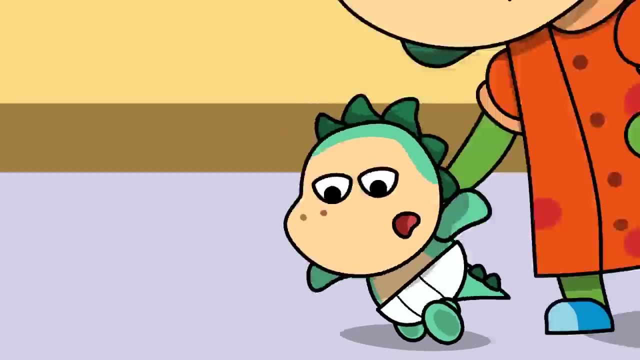 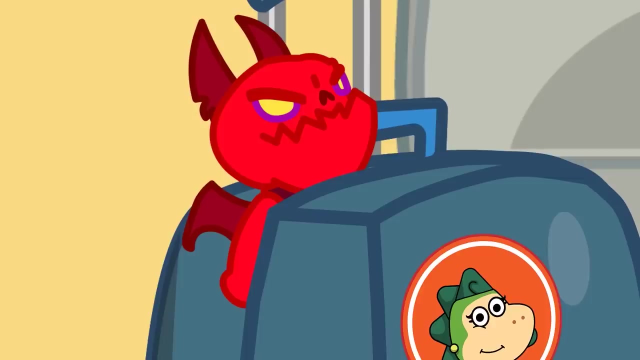 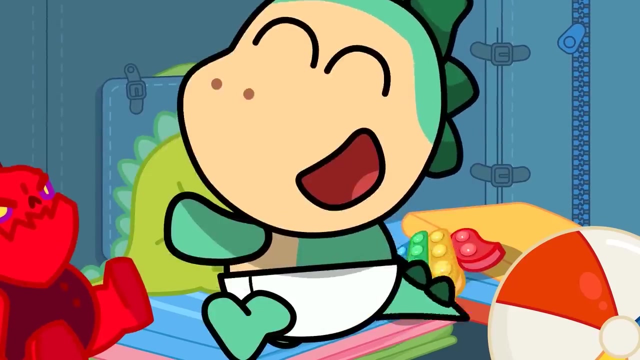 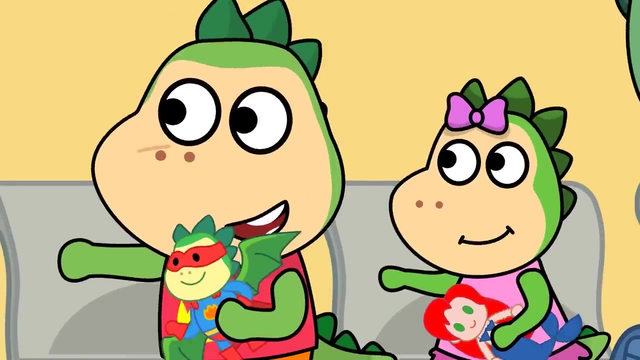 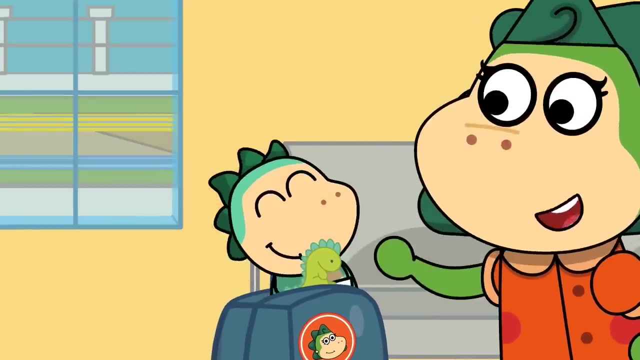 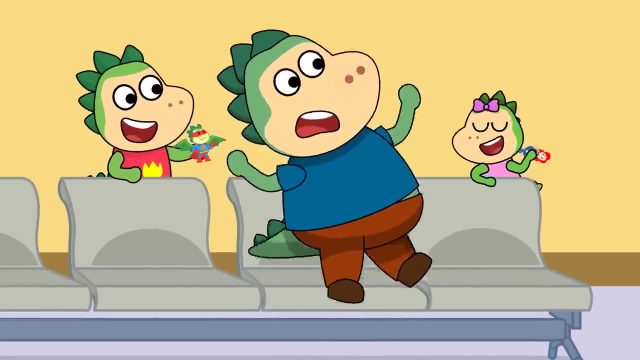 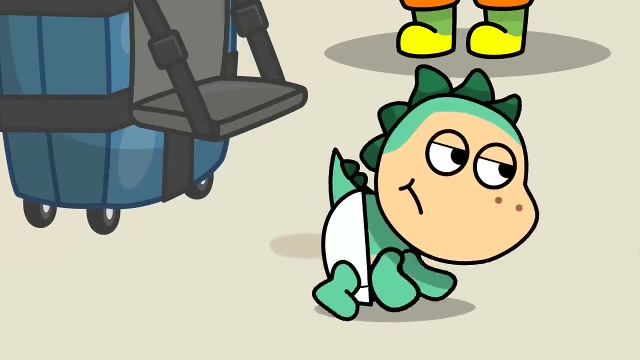 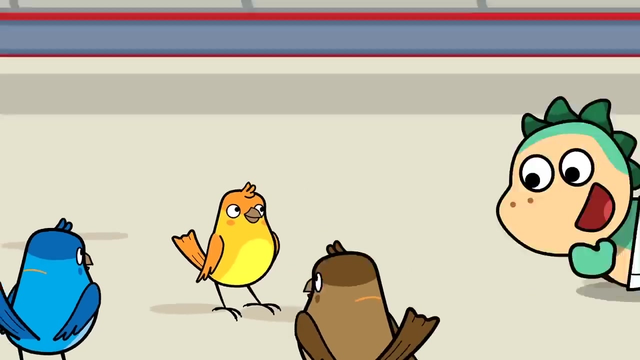 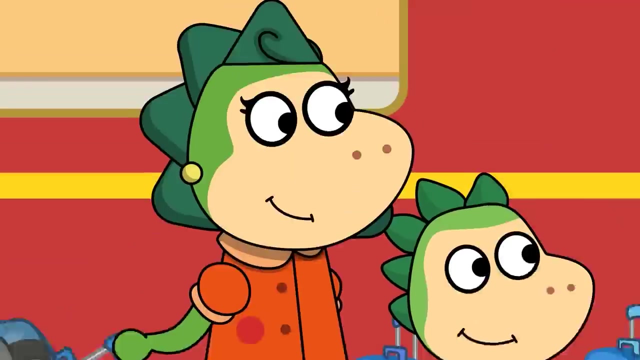 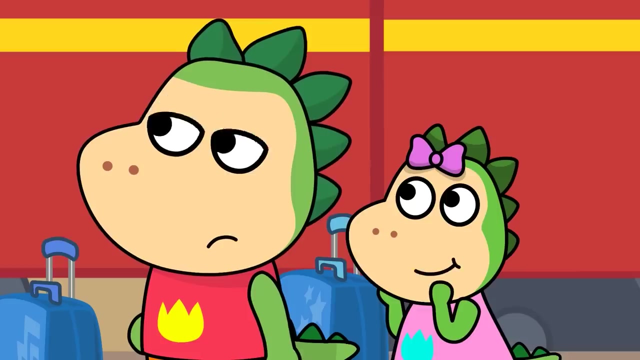 Oh, Ah, Ah, Ah At Ah, Ah, Ah, Oh, Oh, Ah, Ah, Ah, Ah, Ah. Oh, He's in the suitcase. What a safe place you found. Our train has already arrived. Wake daddy, Wake up. Train is leaving. Morning Goodbye, little one, We're leaving. Mom, the bird's telling us something. 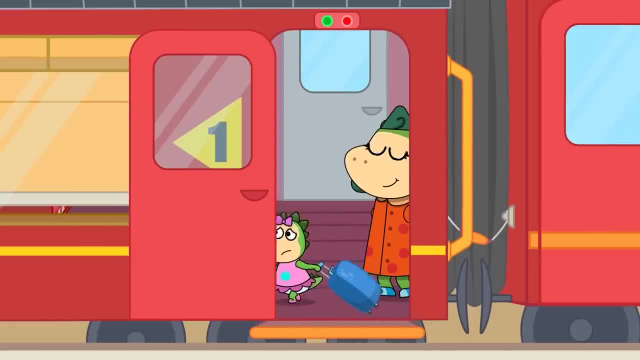 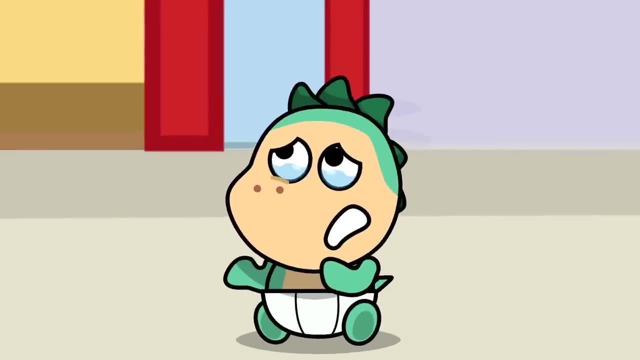 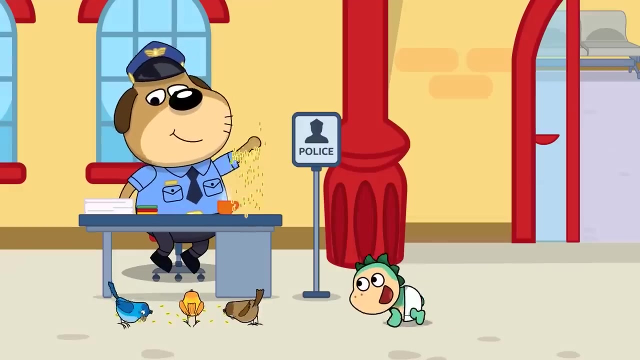 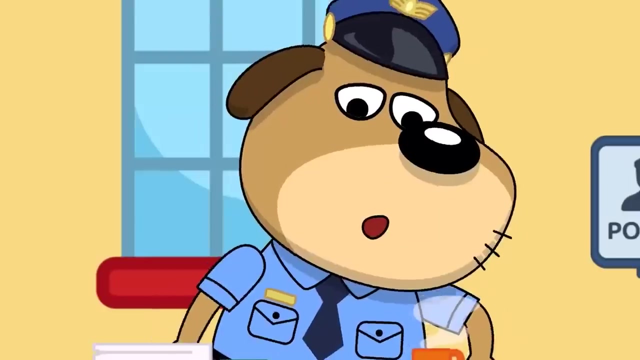 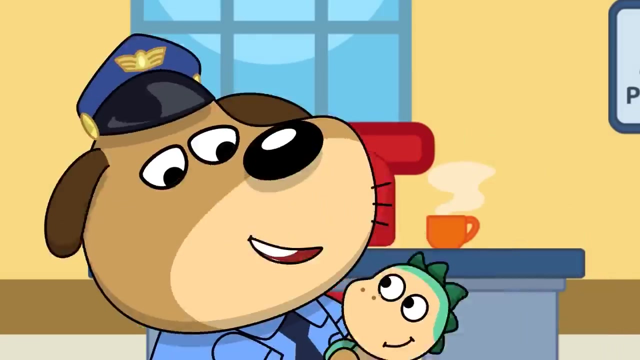 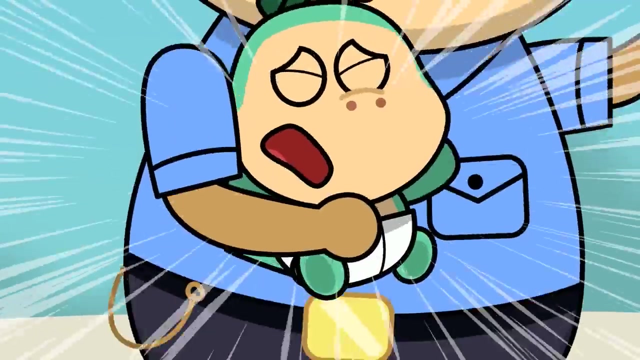 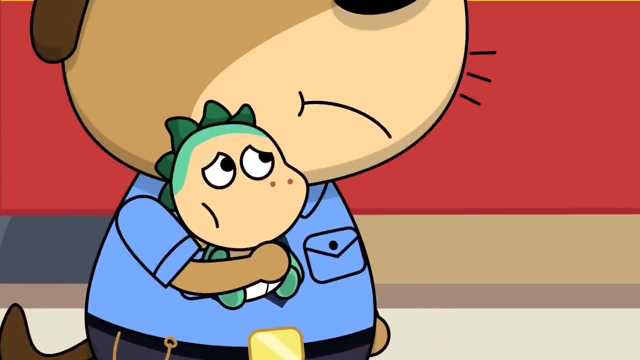 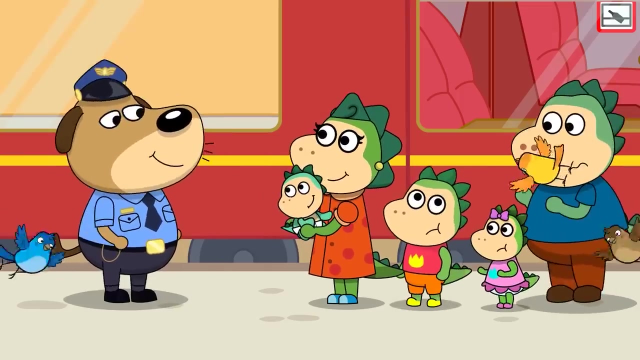 Kids come. We don't have much time. Hi Hero, Where are your parents? Let me help you a little bit. We have to stop the train. Stop the train. Thank you, Mr Woof. Glad to help you, ma'am, And thank you, birds. 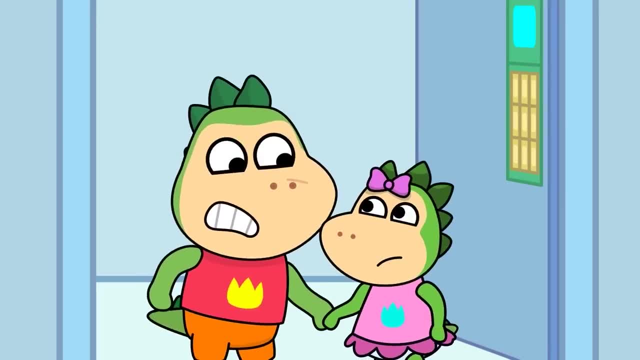 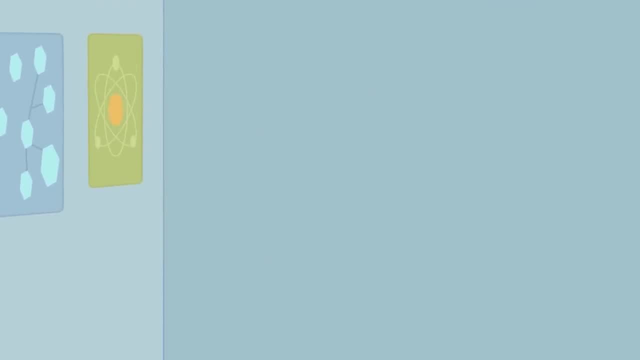 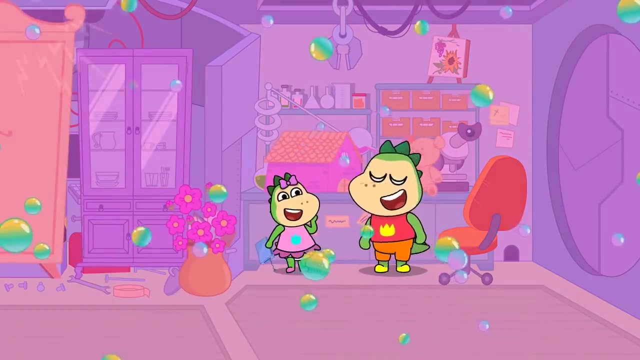 Bye, Sparkle. Nothing to fear here. I'm just testing my new invention. It's an invisible clock. Look, The professor is gone. I can have a look around. The room is pink Sparkle. I'm invisible, but I'm still here. Please push the green button. 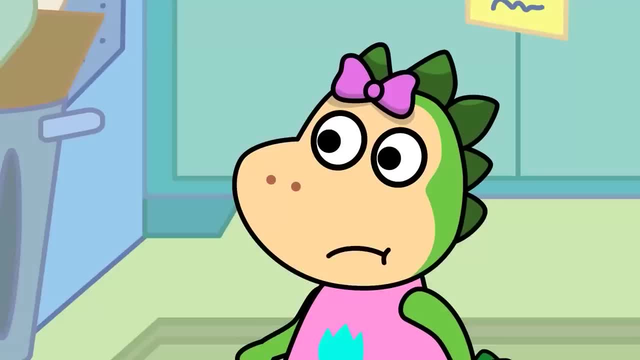 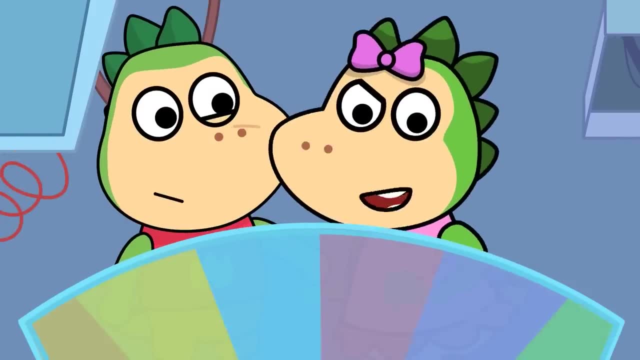 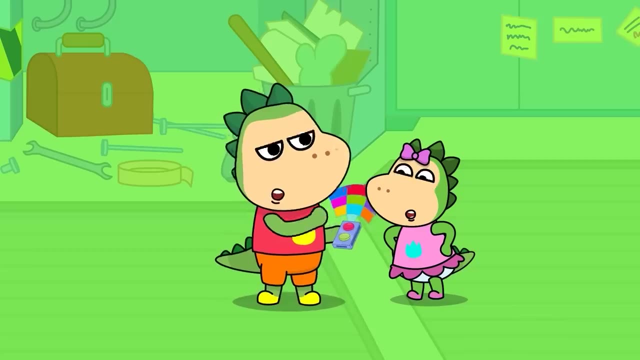 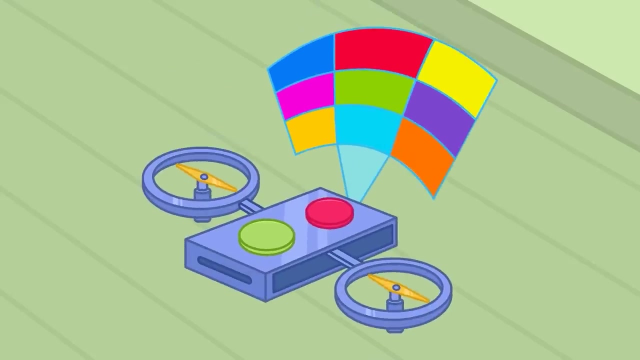 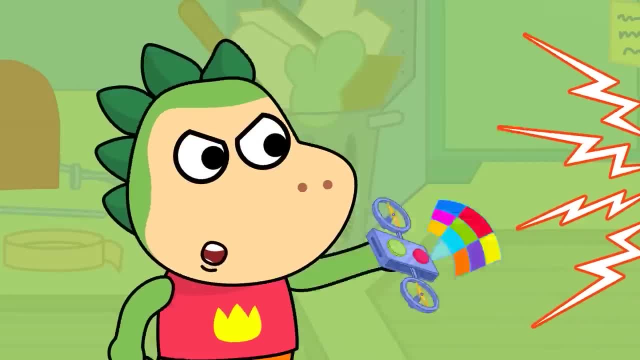 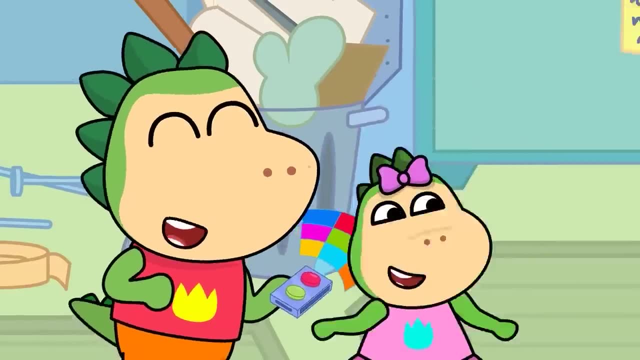 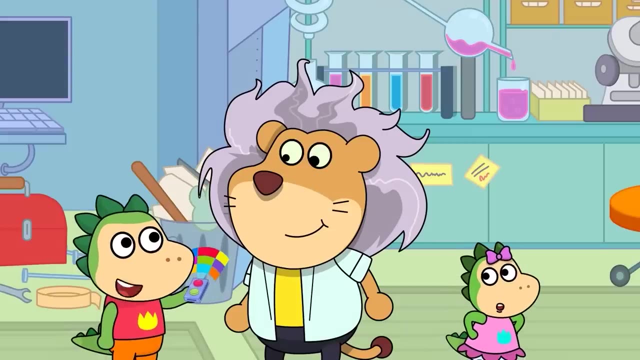 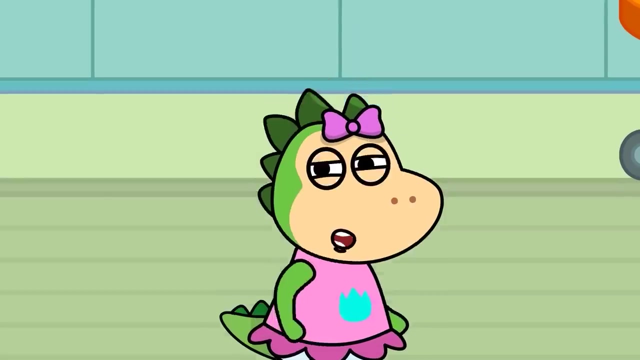 Hello, hello, hello. Press the top button to restart it. Hooray, That was crazy, but I'm glad you were able to make it. stop Here, Professor Roar. Thank you, Spike, Follow me. Let's make sure this won't give any trouble again. 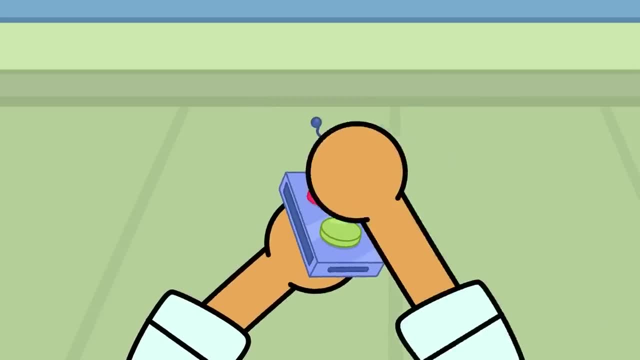 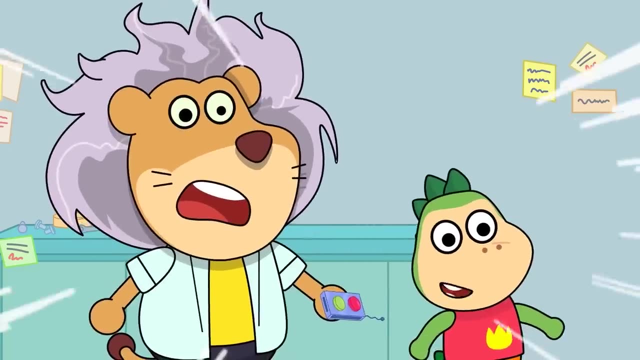 Oh, Hmm, Hoo, hoo, hoo. Oh, Now it won't be so funny. I'm going to put it back in the bathroom. Where's Sparkle? Where is she? Oh, no, she's invisible. Now, where can she be? 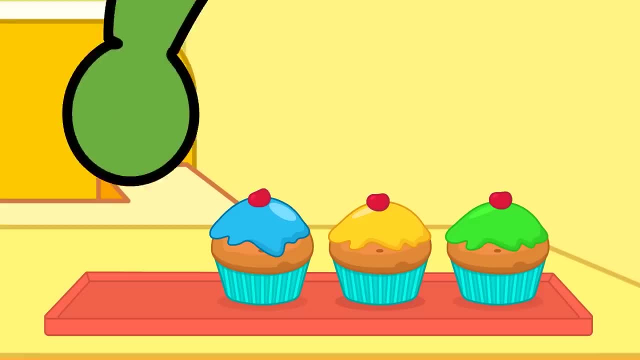 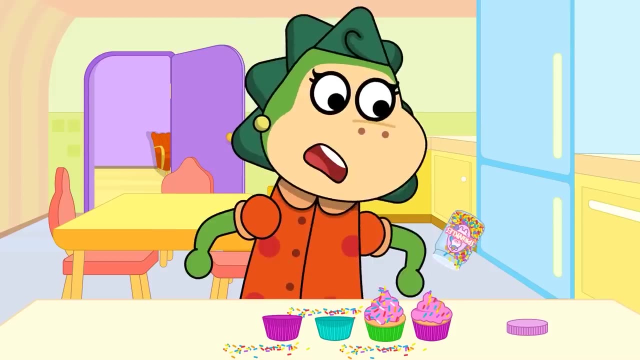 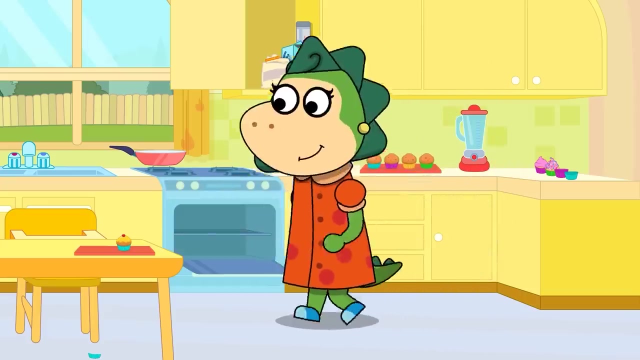 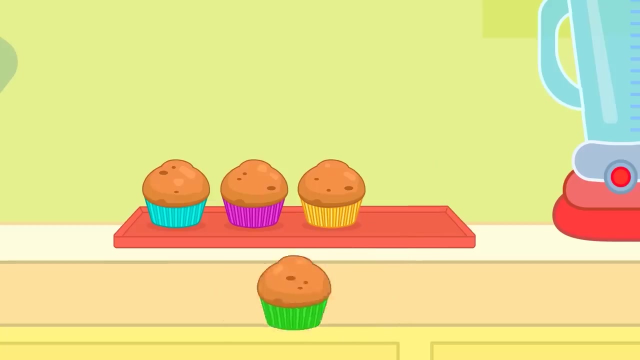 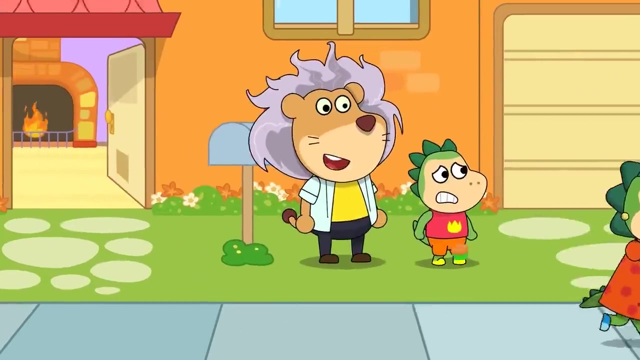 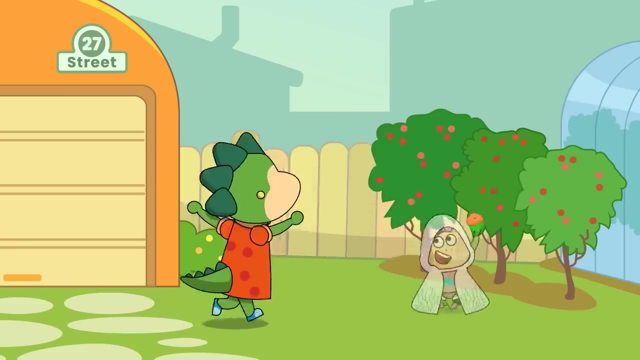 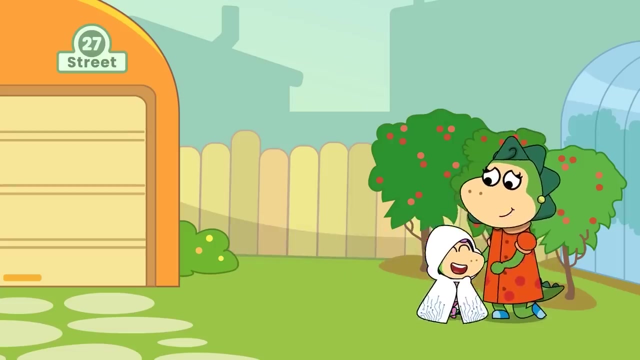 Hmm, green, yellow, blue, red One is missing. What's happening? There's a ghost in the house. Well, Spike, it's time to help your mum and sister. Hmm, Hmm, Sparkle, it was you. I was just joking, Mammy. Oh, sweetheart, you scared me so much. 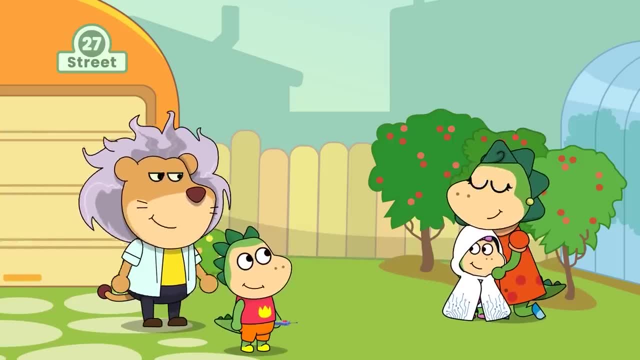 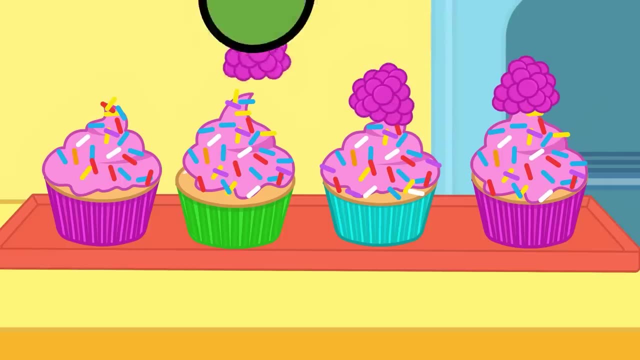 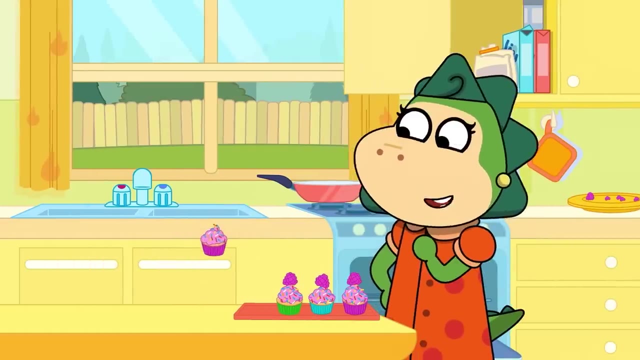 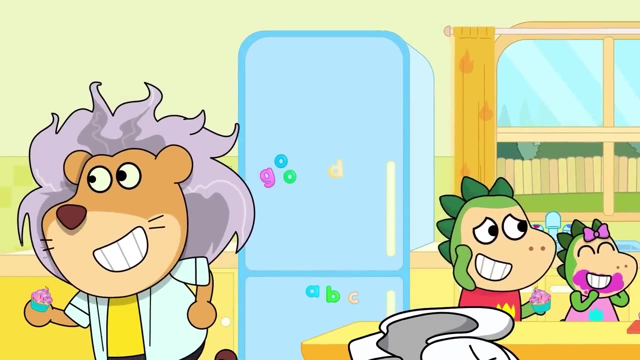 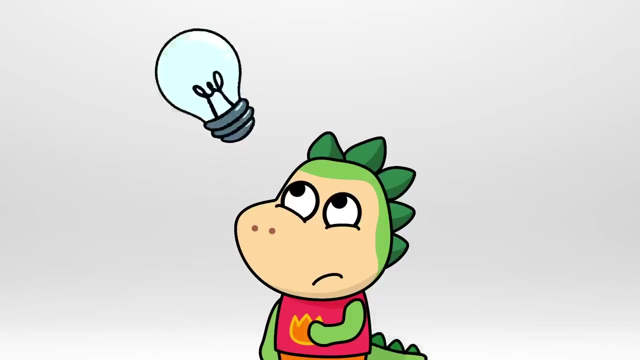 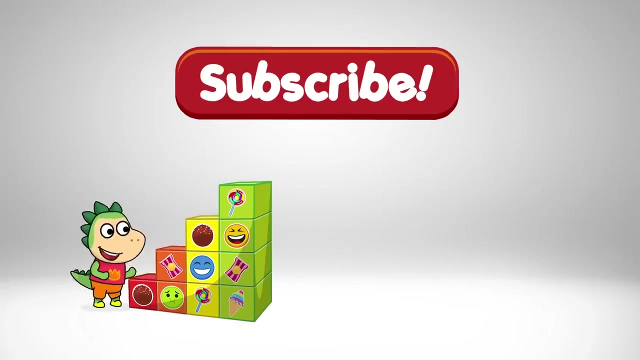 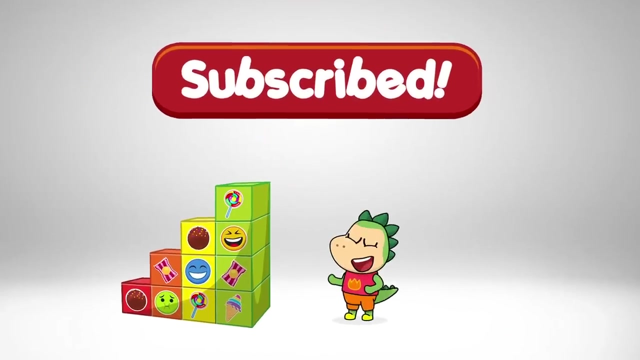 That's totally my fault, Mrs Dragon. Another invention, you know. Oh, Hmm, Huh, Huh, Again, Sparkle. I'll call Professor Roar. Please don't call him. I won't do it again, I promise, Stop.